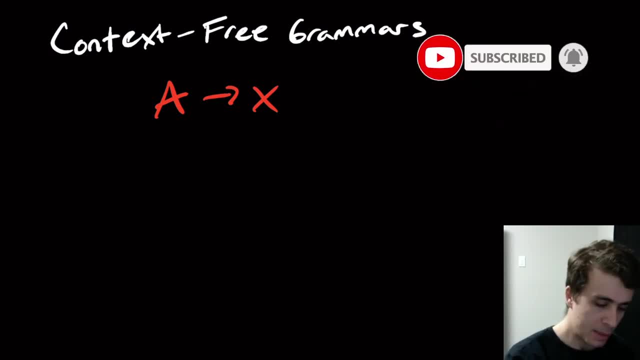 one variable with a bunch of other stuff. But this is kind of irksome If we look at this right here and we say, well, that could be anything right. So is there anything that we can we anything that we can do about it? I said anything three times just there. Is there anything we can do about this? 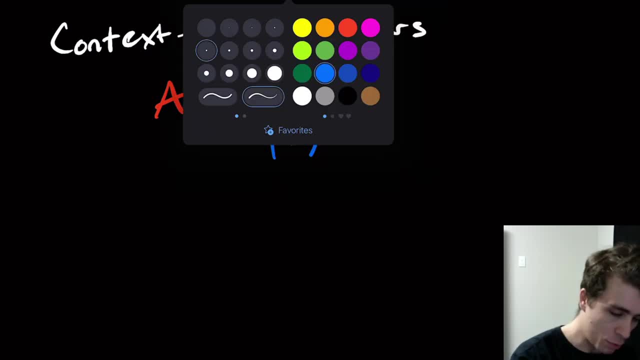 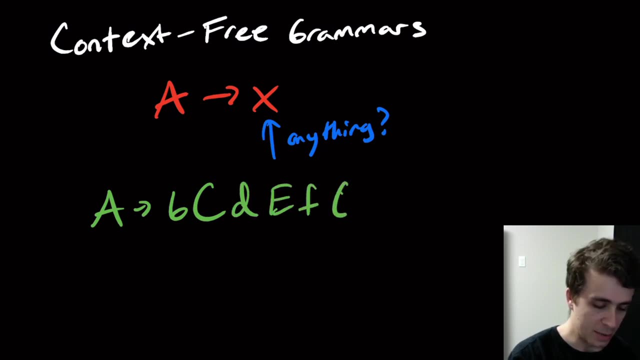 Because if we look at a really complicated rule, for example- so like a goes to b, capital, c, d, e, little f, g, little h- It's so like a really complicated rule with that is a mixture of variables and terminals, We can't really reason very much about what this rule can. 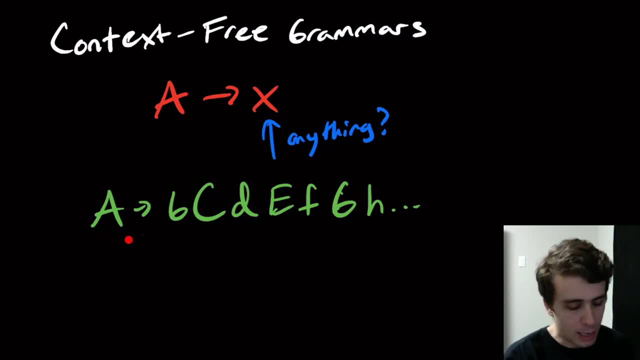 really do. So we could try to. We say, oh, it starts the b, but then it follows anything that c can make, then the terminal d, then with the variable e, whatever it can make. So we could try to figure it out. but when it's in intermersed with a whole bunch of other variables and other rules, even of 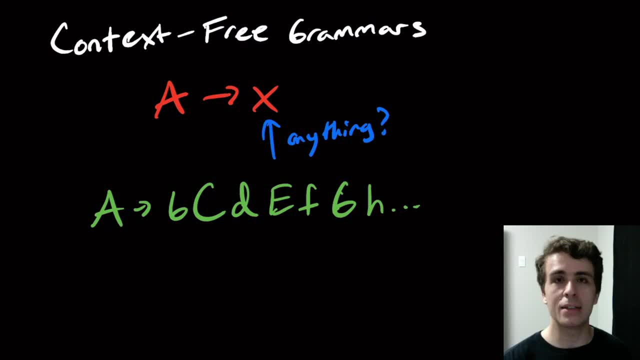 a. this could actually be quite cumbersome And actually what we'll prove later in later videos is that there are certain properties of context-free grammars we can't even decide or figure out with an algorithm, purely because we can have things that are much more complicated. 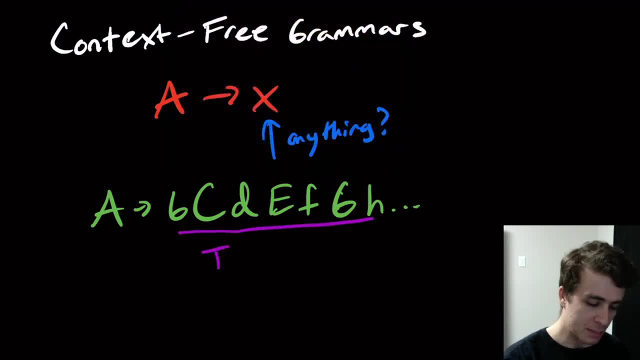 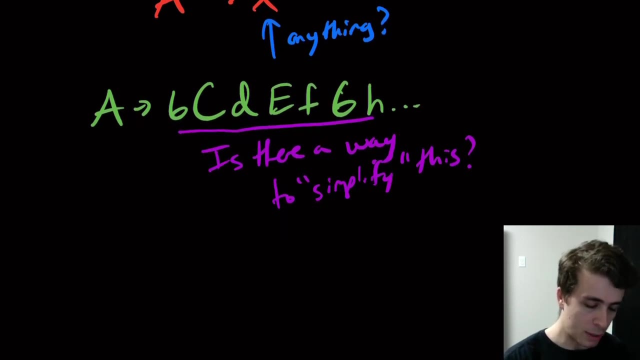 But is there anything that we can actually do about this? So, is there a way to simplify this? Okay, if there is, that'd be great. So that's what we're going to talk about today, which is something that you all are probably familiar with, which is something called. 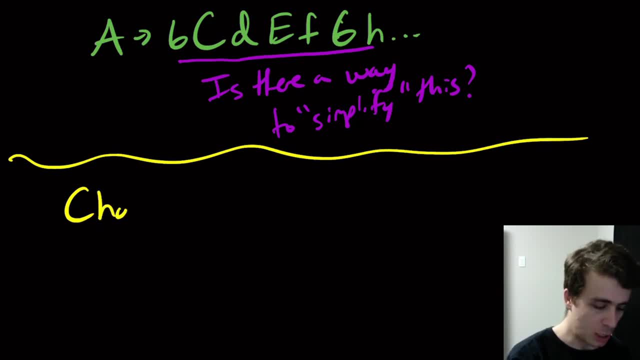 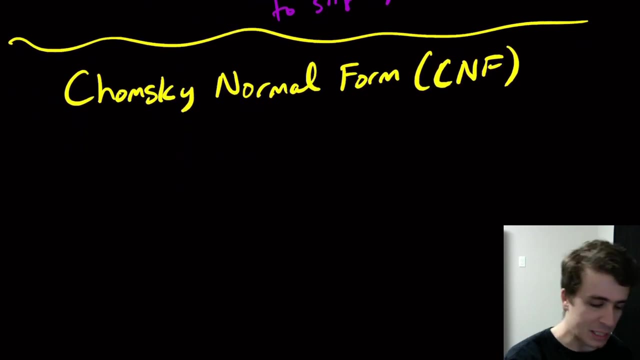 not con, It's Chomsky. Learn to spell Ryan Chomsky, normal form, And you're probably in a class. you probably are learning about this right now and you you probably know the basic idea, But in case that you don't, Chomsky normal form is restriction on what that right-hand side can be. 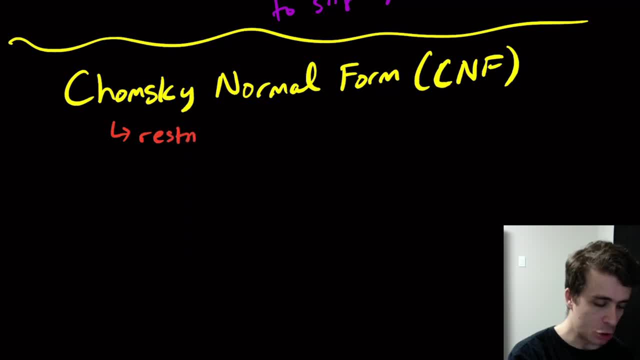 So, if you don't know anything else, it is a restriction on the right-hand side. So what is the restriction? Well, there are three things that are true in a grammar that's in Chomsky normal form. So the only rule that can make: 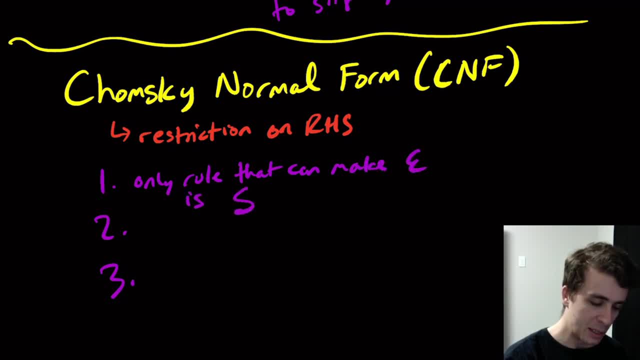 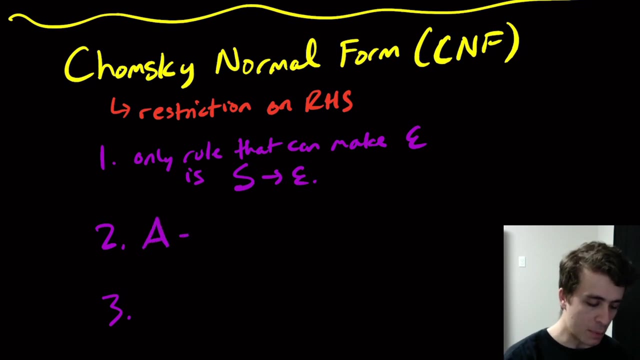 the empty string is the start variable can make it. So that's the only rule that can make it. No other variable can make it. Only this start variable can make it. We could have any variable will make a single terminal and nothing else. So we enforce here. 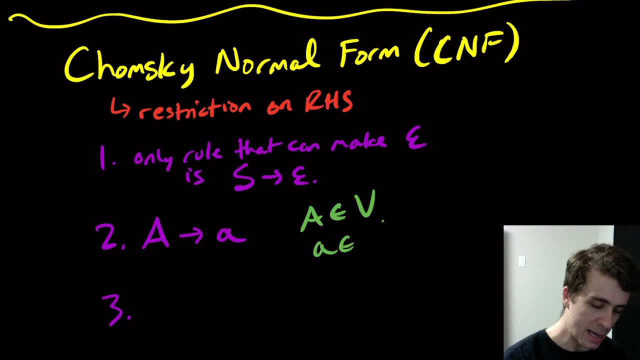 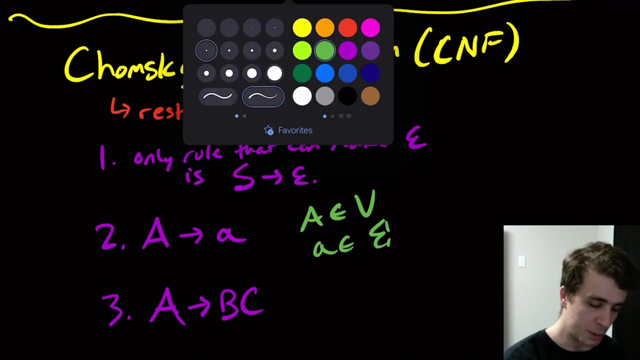 that a is a variable and a is a single terminal Or what we can have, because if we just restrict to these two, then we're still in regular grammar land. we want to get something for the context-free languages instead. so the other type of rule that you can have is variable a makes two variables, So 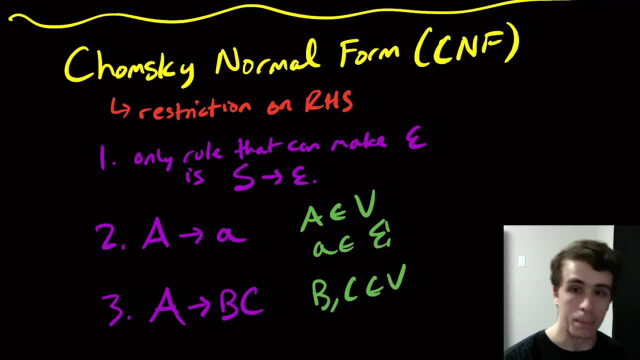 here B&C our variables. but we're not done yet. We are also going to require that B and C are not the start variable. Okay, so this variable here is an empty term and we cannot have any variables right now If we make a part of it and add the first one to it, So we can avoid it If a variable is empty. 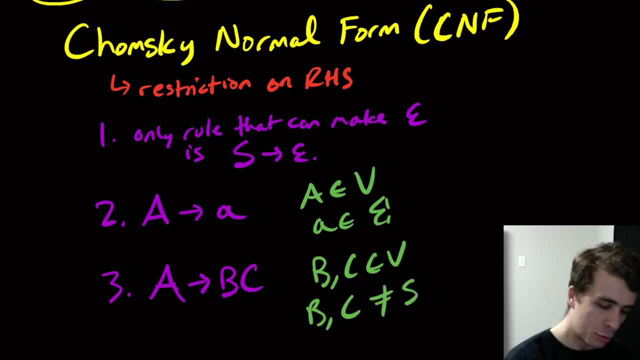 that does get removed from the rule. So just get the first partner without any variables right in. Okay, so you have extended value, Alright. so if you don't have any variables right now, then Okay. so you may think: okay, who the hell created this? 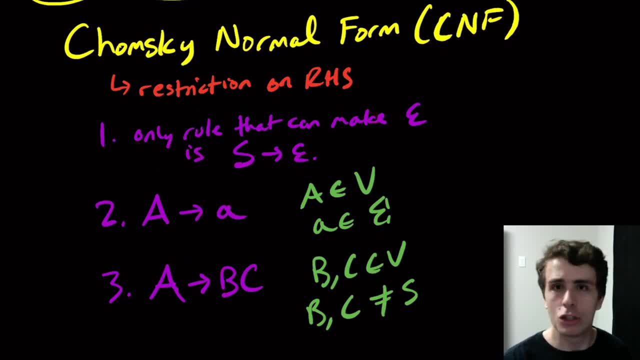 Who created these three rules And why would you even care about such a thing? Why would you want something like this? Well, here's the thing. The rule types are really simple. Only one rule can make the empty string, And we saw that with the ambiguous example. 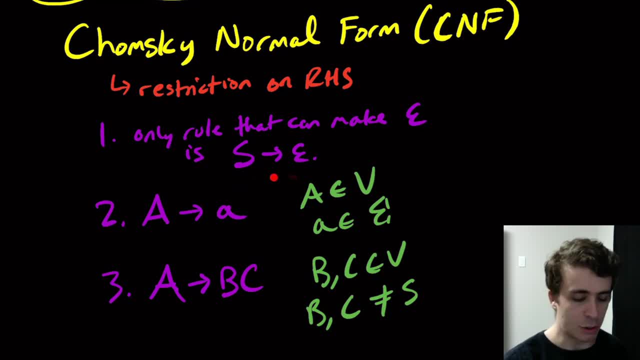 where there are many ways that we can make the empty string. If there's only one way we can make the empty string, that's fantastic. And look at the other rules. You can either have one terminal or two variables, nothing else. You can't have a mix of them. 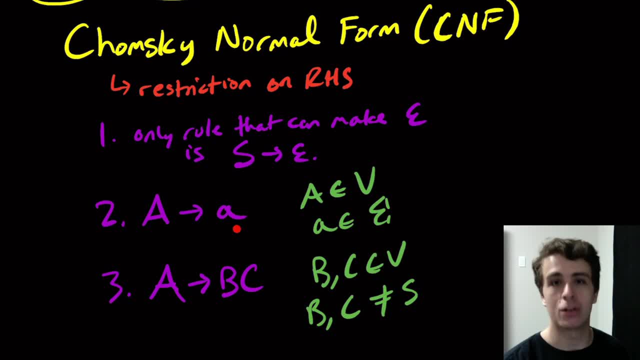 You can't have more of them. You can have just one terminal or just two variables, which is kind of cool. So it makes the grammar significantly easier. But there are actually some things that we'll talk about at some in-depth and later videos. 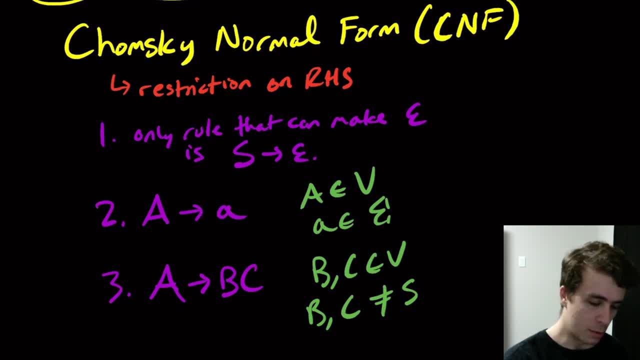 that show the true power of Chomsky Normal Form. This really is one of the most important things about context-free grammar is because it gives us so much information. But you may think, okay, well, certainly I can make a grammar like this. 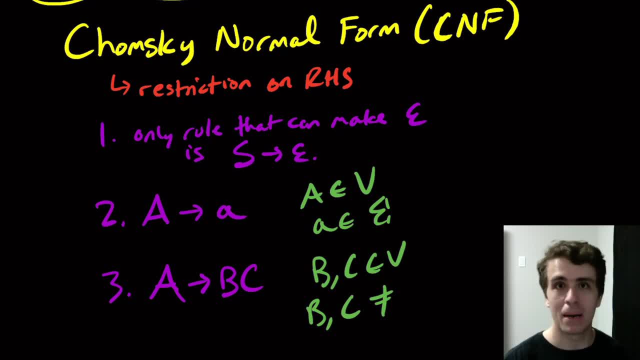 Hell, I can just copy these rules down and bada-bing, bada-boom, we got it. But is it the case that we We can make any grammar into any context-free grammar, into one that's in Chomsky Normal Form? 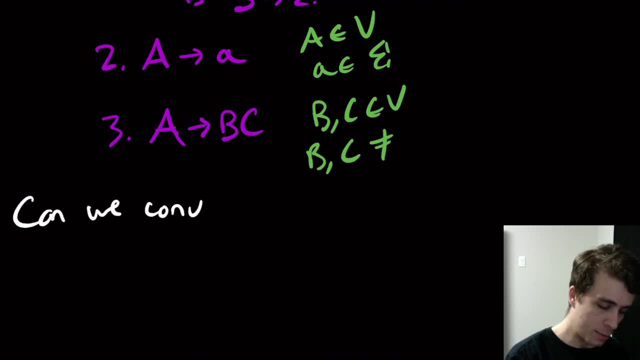 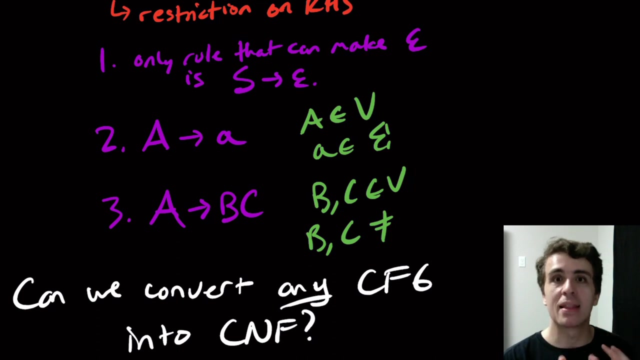 So can we convert any context-free grammar into CNF? Can we do it to any grammar? So is there a way that I can keep the language of the grammar exactly the same but have a version of it, A version of it that's in Chomsky Normal Form? 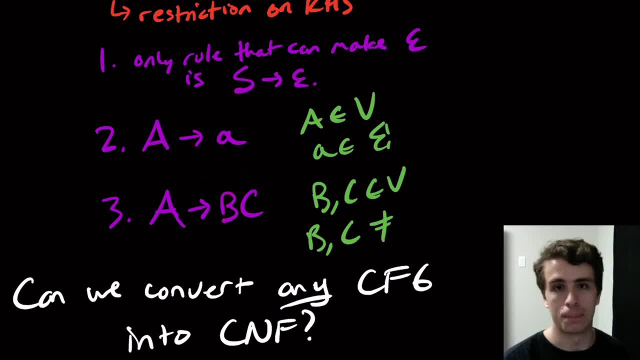 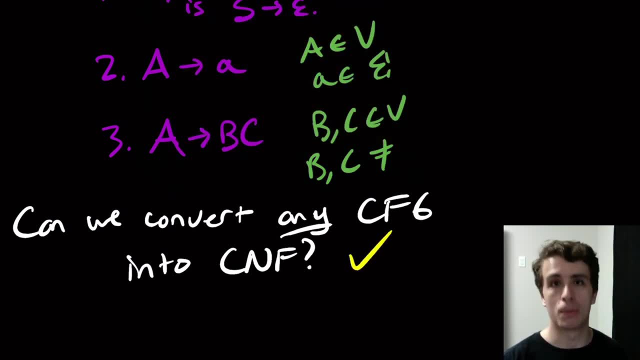 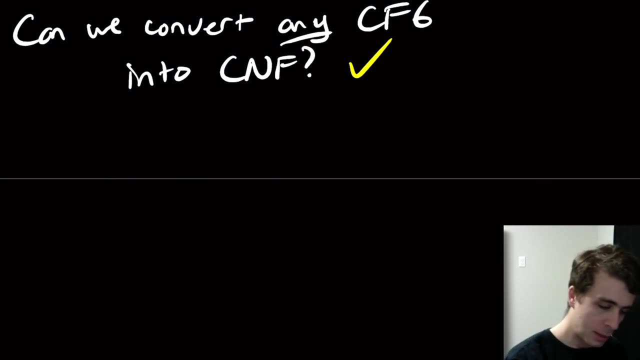 Because I can certainly make a grammar that isn't in Chomsky Normal Form, And what we're going to answer today is in the affirmative: This is possible, And, moreover, there is an algorithm to do it. So how do we actually go about doing this? 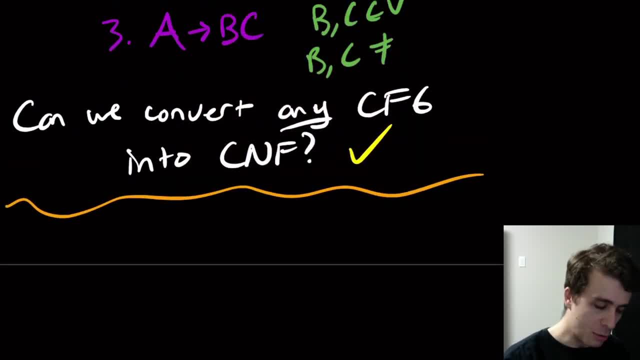 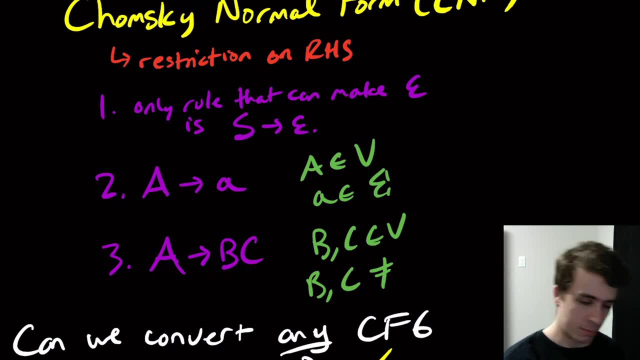 So let's actually look at these three rule types again. So this one says that the two variables on the right-hand side- Oh, I forgot to put the start variable. Oops, That was my mistake, That these two variables can't be the start variable. 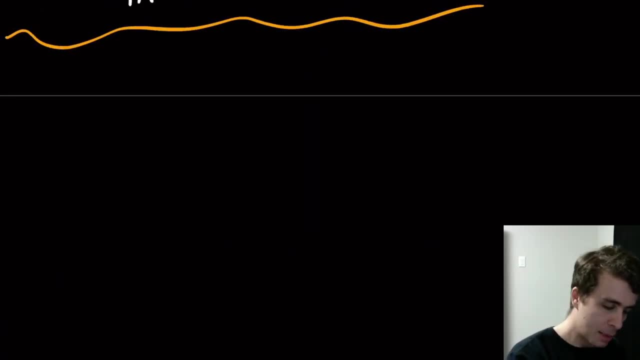 So one thing that we can actually do right off the bat is to ensure the start variable and not on- oops, not on the right-hand side of any rule. And how can we do this? So let's say that S was the original start variable. 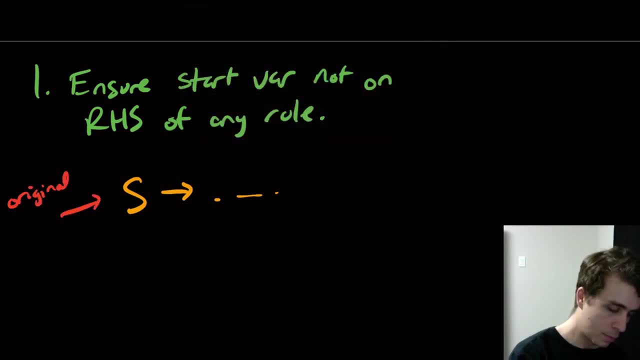 So this guy right here is the original start variable. Well, I don't know anything about the structure of the grammar. Maybe there is some weird rule down here where it has S, B or something, where one of the two variables is on the right-hand side. 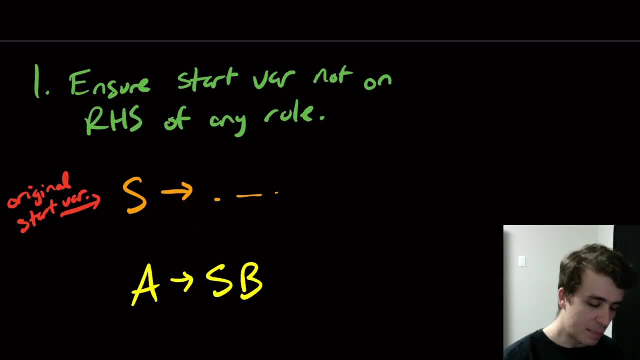 That is the start variable, And maybe that is the case. We're just gonna handle the case entirely. We won't even think about what the grammar even looks like. So how are we gonna fix this? What we're going to do is make a brand new start variable. 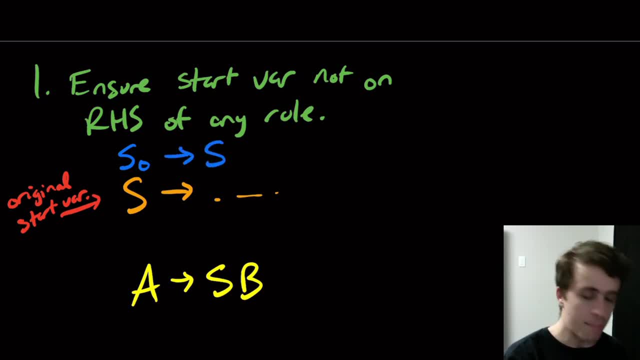 I'm gonna call it S zero and have it make the variable S. So this guy right here is the new start variable. So this guy right here is the new start variable. So this guy right here is the new start variable And what we're going to actually make sure of. 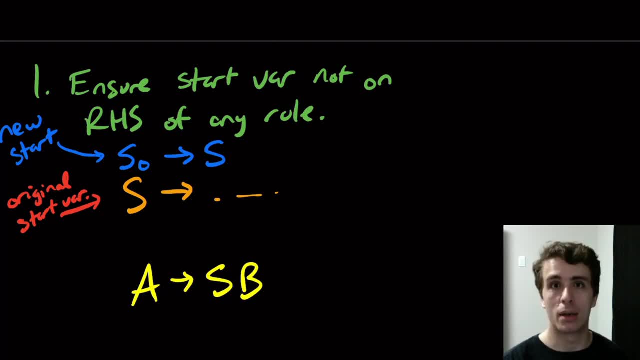 is that we don't change the language of the grammar at any step. So in this first step, right here, do we change the language of the grammar? And I argue no, Why not? Well, suppose that we can make a string of terminals. 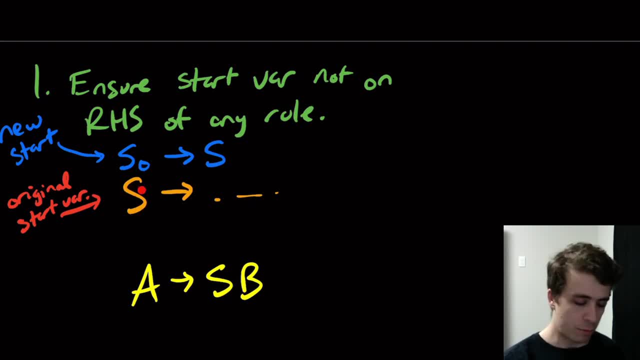 from this start variable right here, from S. Well, how can I make the same string from S zero from S zero? Well, it's only rule is to go to S, and that didn't make any terminals in the process, And then we can follow the same rules. 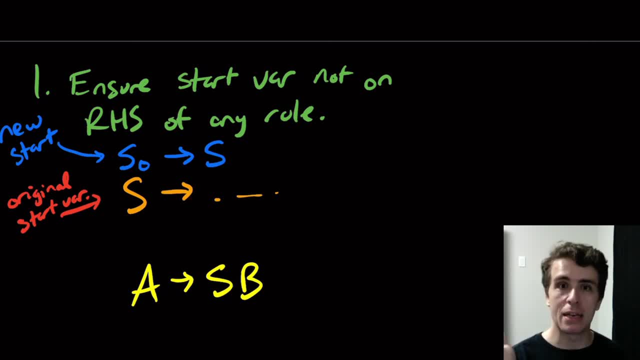 we would have done with the S one. So that shows that the original grammar, whatever it make, the new grammar also makes. But what about the other way? If the new grammar makes something, does the old grammar make it So in the new grammar? 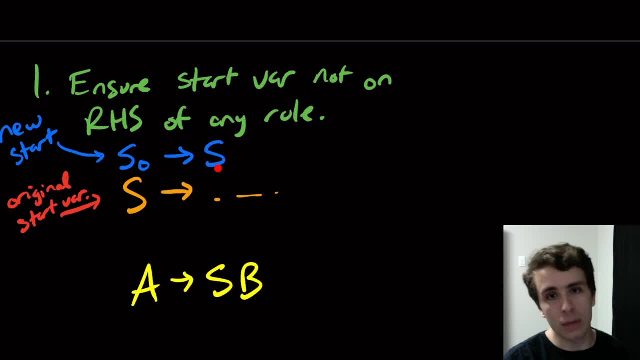 we have to start with the start variable, And it's only rule is going to the original start variable and then S will make something Well in the derivation. what we can do is just chop off this application of this rule and then basically just start it off at this variable, S. 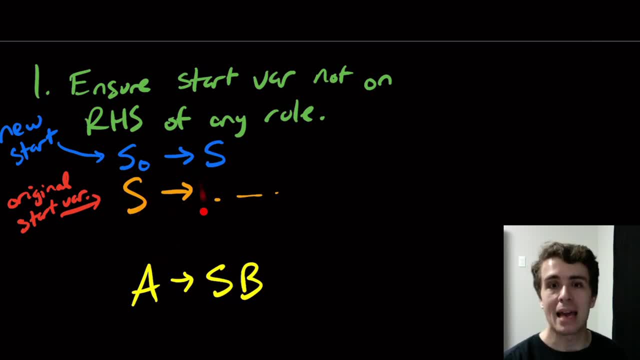 which was the original start variable, And so we get a derivation in the original grammar. okay, So this tells us right here that we don't actually change the language because this rule right here that we have to use in order to generate anything 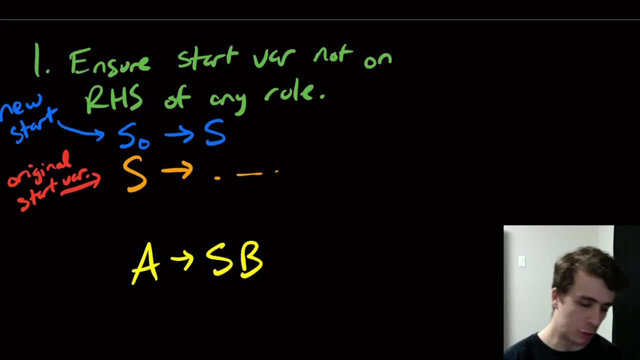 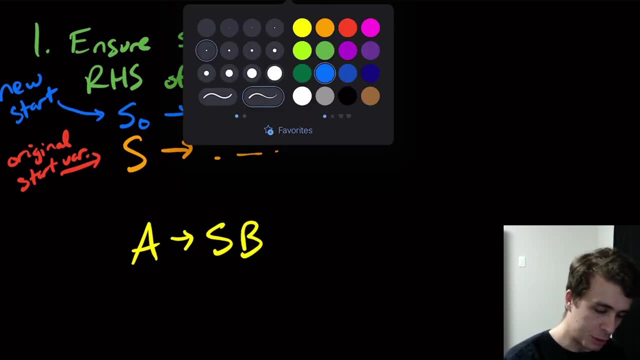 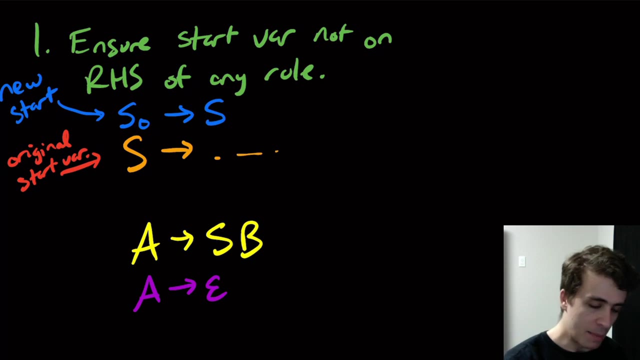 doesn't make any terminals And that proves it, which is pretty cool, Okay. well, what about some other rules? So maybe we could have some other variable, or maybe A does this. A is a bad variable, makes the empty string. 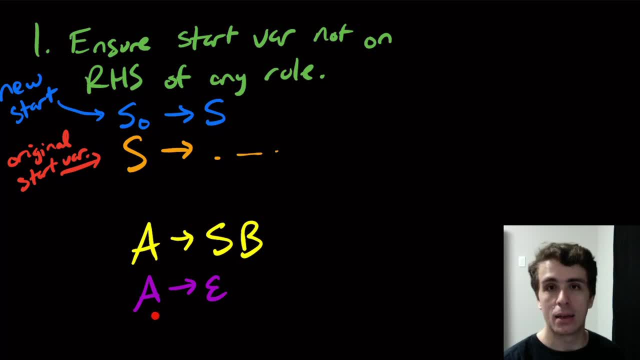 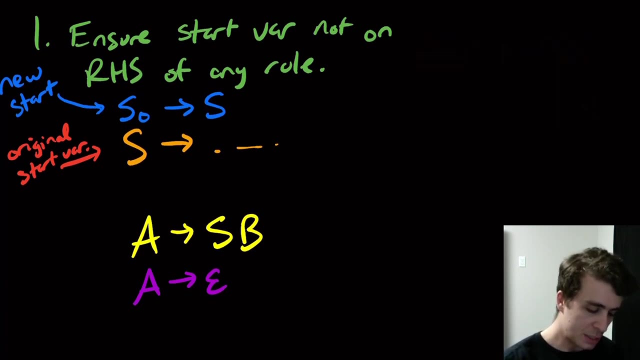 Well, the rule says that anything if we are going to make the empty string, only the start variable can make it, not some other variable. That's what the rule said. So how do we fix this? This is actually considerably harder, because what if we have, like, some variable B? 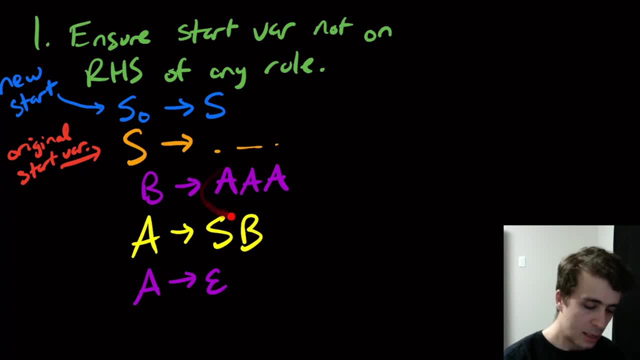 which is going to make three A's, right. So maybe this variable B can also make the empty string, because each of these of these individual a's, by this rule down here, can make the empty string. so I, so we can actually infer that b makes the empty string too. so what we want to do is to figure out: well, how do we? 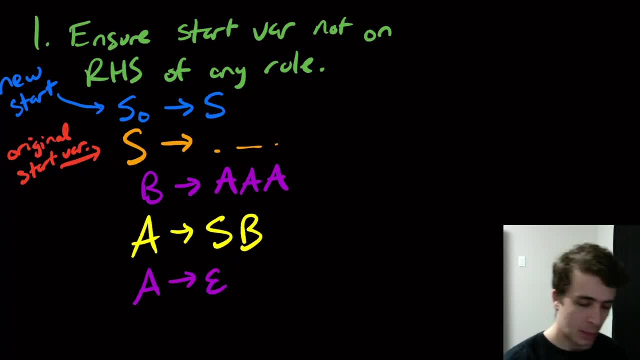 account for this. well, I gotta get rid of this rule. but if I just say, oh, I'm gonna chop off that rule, that's gonna change the language of the grammar because it there may be some other rule right here. let's say b goes to little, a, big a. and if we chop off this rule and let's say that a capital a. 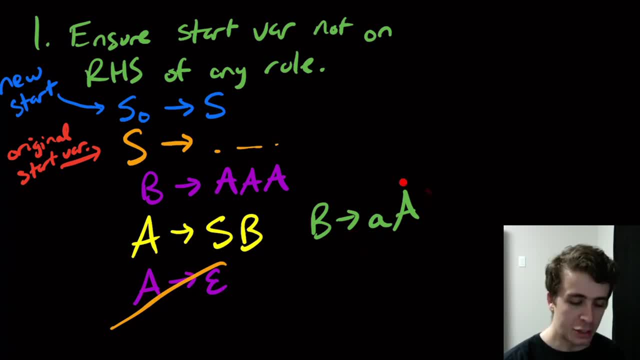 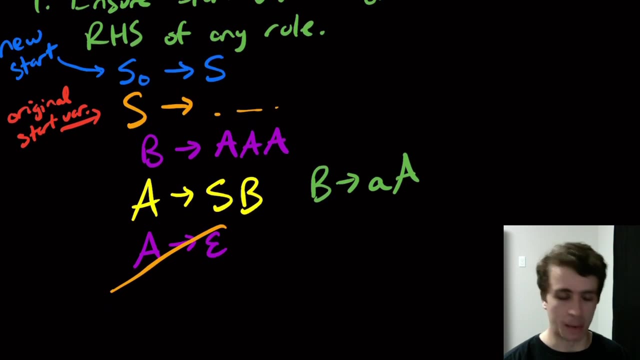 doesn't make anything else, then this rule is completely useless, because the variable a is not going to make a terminal anymore. or it may not be completely useless, but it could change the language of the grammar for sure. so we got to be a little bit smarter about this. 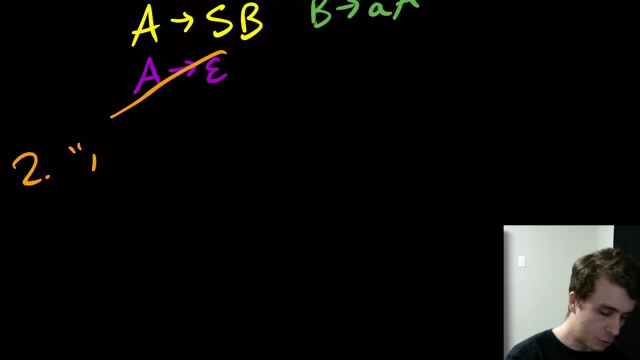 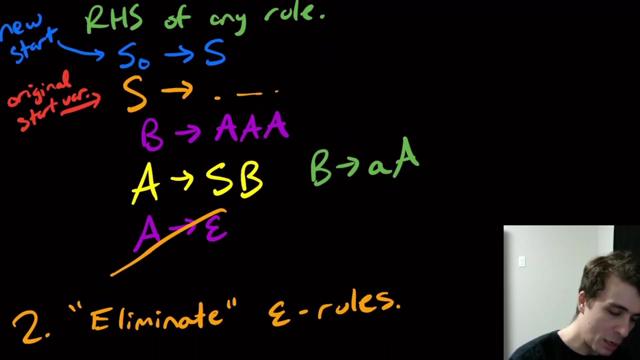 so how are we going to account for this? So the way I write it is I'm going to write eliminate, in quotes, epsilon rules. So I don't mean literally eliminate epsilon rules, I mean just to strategically get around it and then eventually get rid of them. So what? we can look at this example right here. if I was just so clever. 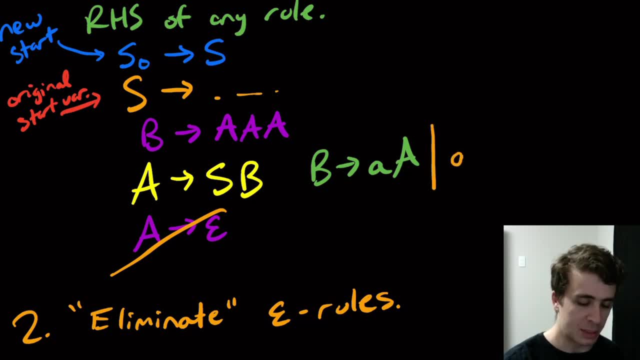 as to say: oh, I'm going to put another rule that says, if the variable a went to empty, I'm going to put another rule in the case that it went to empty. Okay, so I'm basically just: if I did this, I'm. 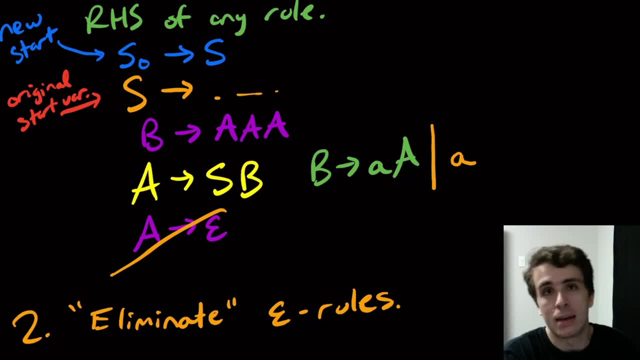 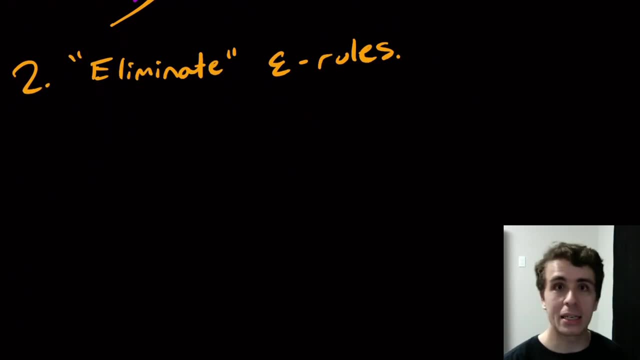 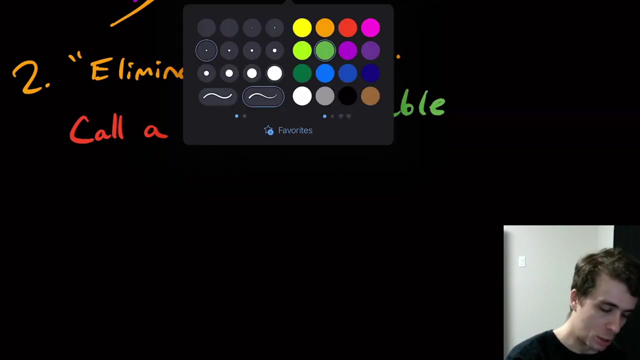 simulating as if the variable a went to empty, even though I'm getting rid of that. So I'm simulating it with a different rule. So that's actually the exact right idea. So we're going to call a variable. it's a term nullable, so that's just a term If and I'm going to call the variable. 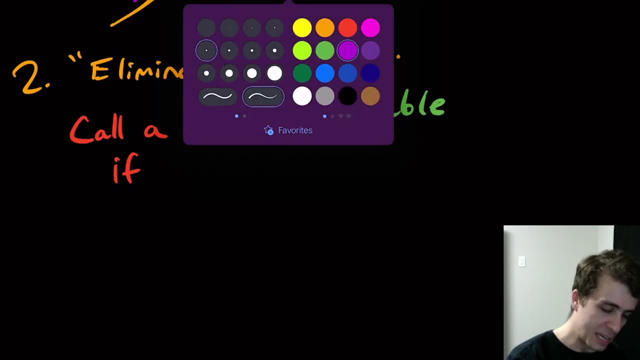 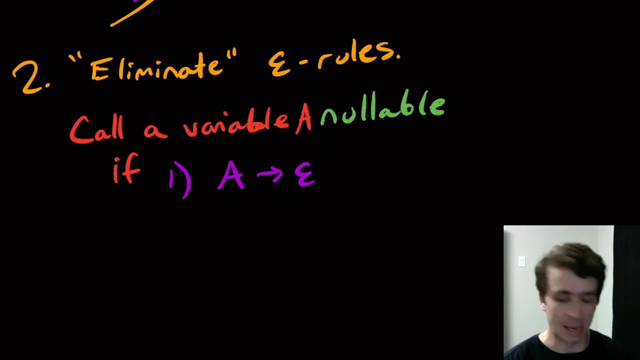 a if one of two things happens: If a makes the empty string directly, if a just directly makes the empty string, so it obviously can make it. or it's the case that a makes the empty string directly, so it obviously can make it. or it's the case that a makes the. 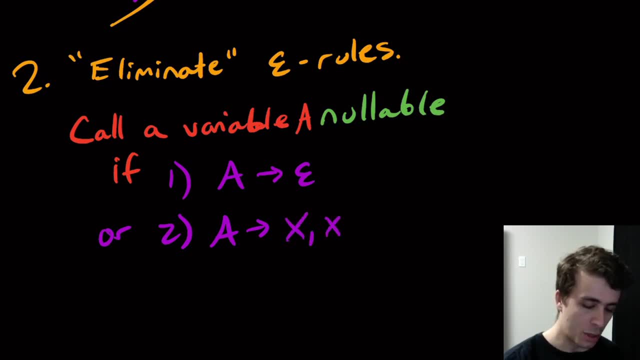 empty string directly. so it obviously can make it. or it's the case that a makes a whole bunch of variables. I'm going to call them x1,, x2, up to xm. but it's just some set of variables, no terminals. 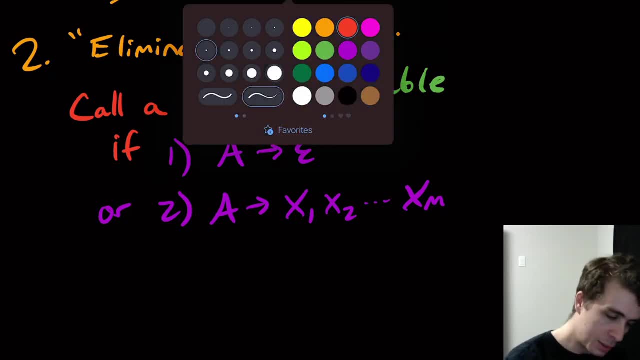 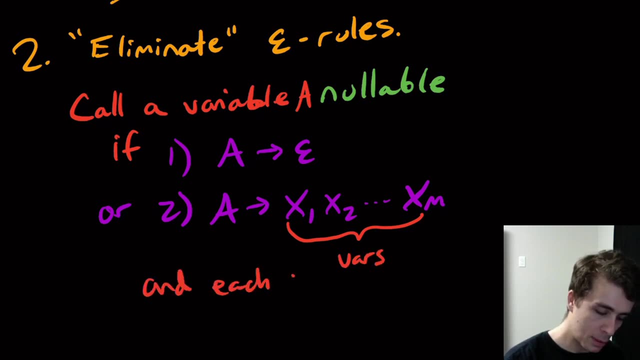 no terminals, just variables. So I should say that all of these are variables and each x i is nullable. Okay, so I'm going to call a variable a nullable If it can make the empty string directly, or it's kind of like an induction proof. This is the base case and this is the inductive case. 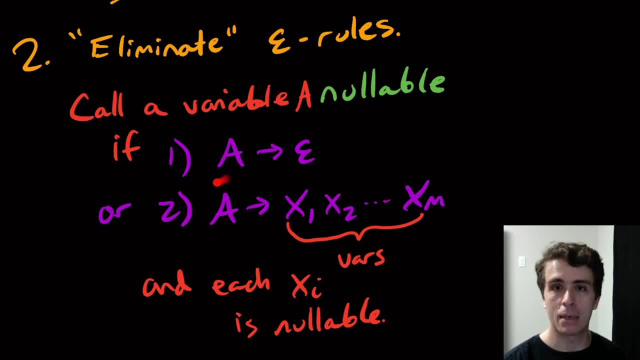 saying: if I have some other variables that are nullable, I'm going to declare a to be nullable too, if it happens that all of these are nullable. If one of them isn't, then I can't declare that a is nullable, because maybe this x2,, for example, doesn't make the empty string at all. and then we 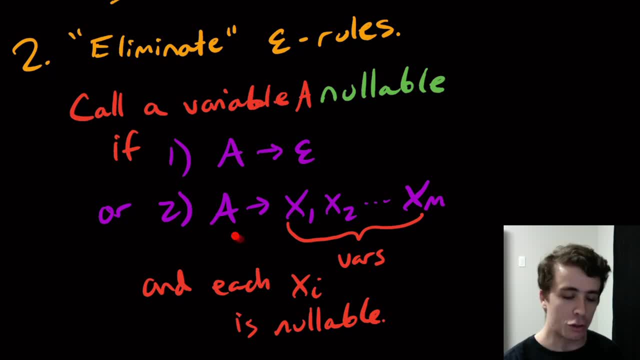 can't declare that a is nullable. So I'm going to call a variable a nullable and if it can make the empty string directly, I'm going to declare that a is nullable from this rule. If there's some other rule that says a is nullable, then of course a is nullable. Okay, so as long as there's some rule. 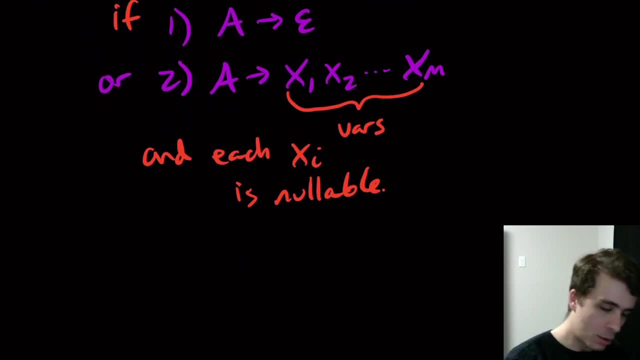 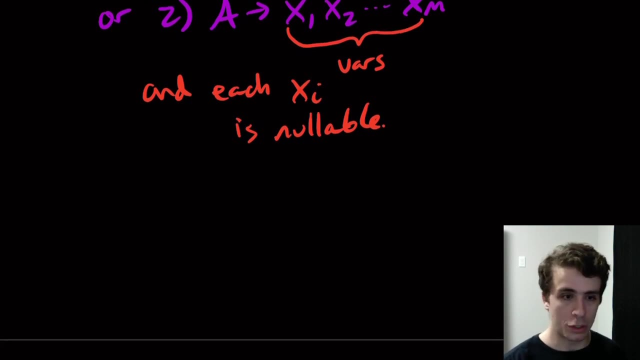 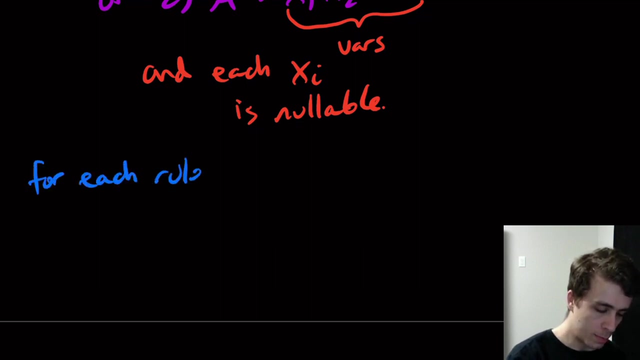 that allows it to make the empty string Okay. so then, what are we going to do here? So what we're going to do is we're going to look at it this way. So if we have some, so for each rule of the form a. 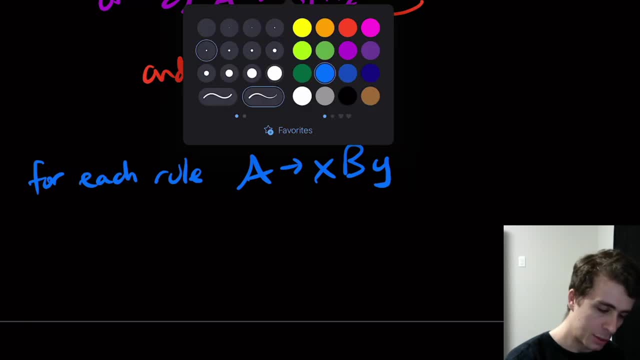 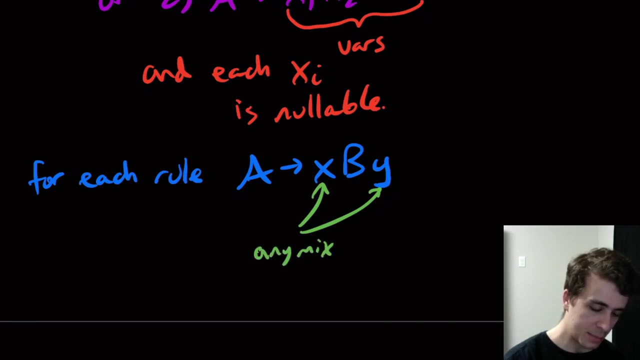 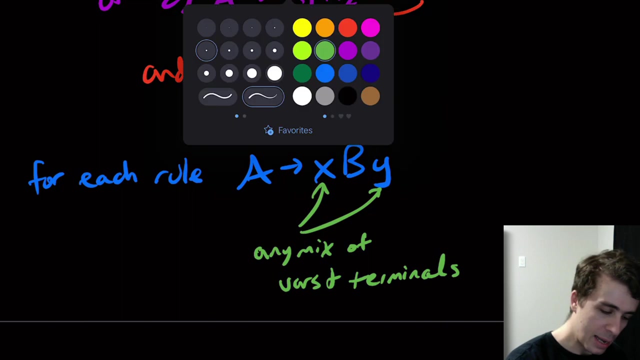 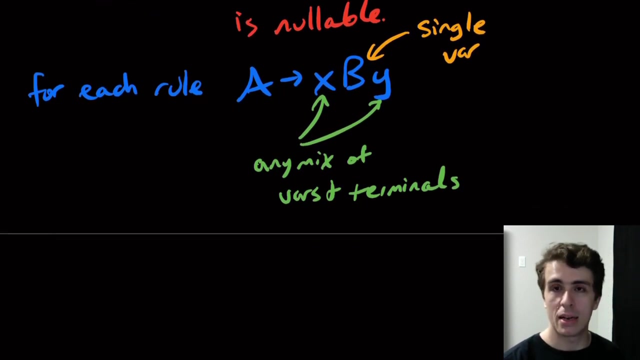 x, b, y. so this is just formal notation to say that x and y are any mix of variables and terminals and the b here is just a single variable. So if we have some rule that like this- and we probably will- so then- and it's the case that if we have some rule that like this, and we probably will- 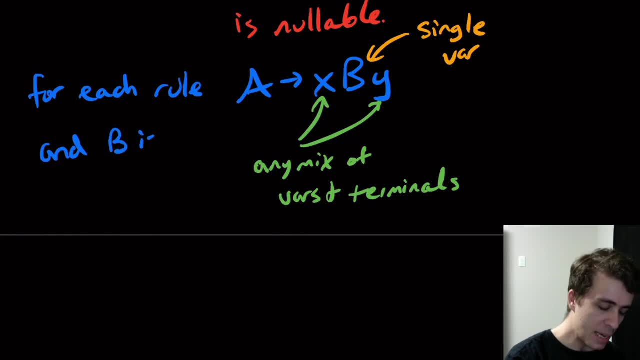 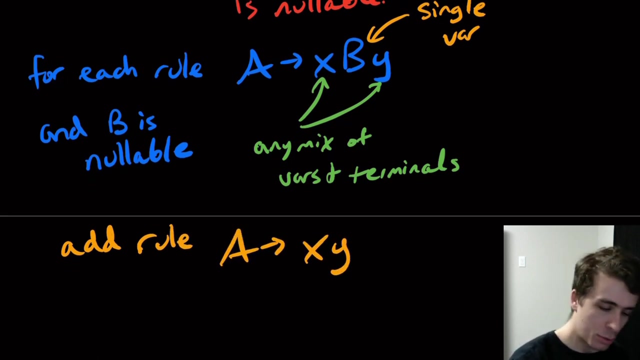 in the case that b is nullable, then what we are going to do is we're going to add the rule: a goes to x, y, Okay, so it's as if I'm taking this b and it's in the case that b is nullable. we're simulating as if. 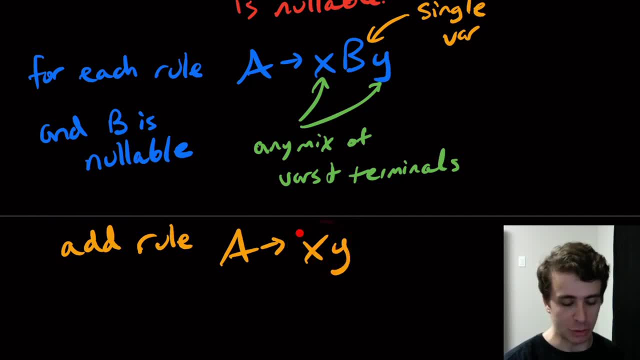 it went to empty, because that's what this rule is. we're not changing what goes before the B here. we're not changing what goes I mean after, yeah, before the B or after the B. so the X and the Y part are exactly the same, even if they have variables, even if they are nullable. 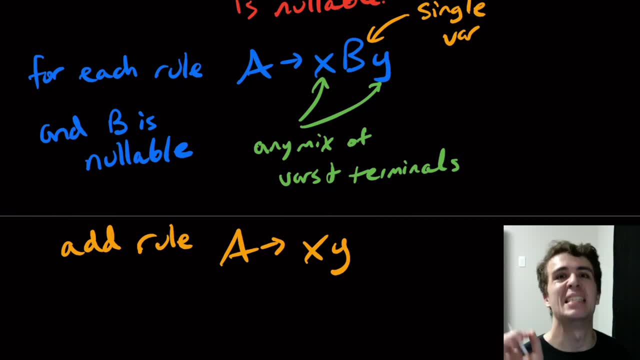 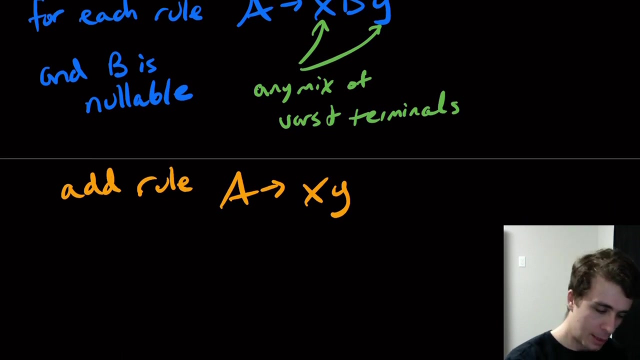 because nullable variables can still make a non empty string. it's not that they only make the empty string, is that they can make it. so we're simulating as if this variable went to empty and we're gonna do this for every possible rule. even if we add a rule, we're going to handle that case as well. some things: 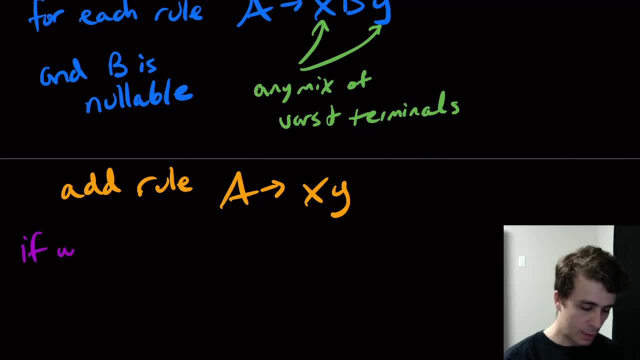 that to note. if we make, if we have some rule of the form, a goes to a, so like a variable makes itself, well, we can just delete that. yeah, because if we have like some no, no, no, no, no variable alongside a, and then we added this rule in case that that variable went. 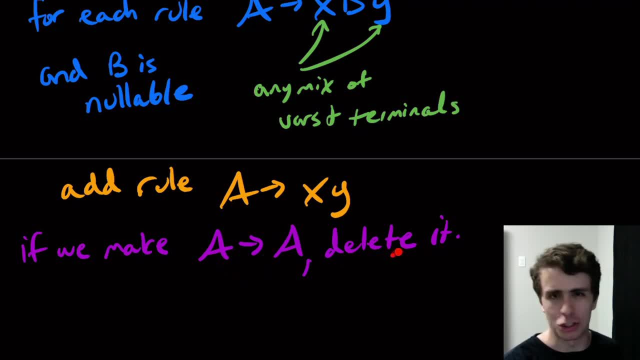 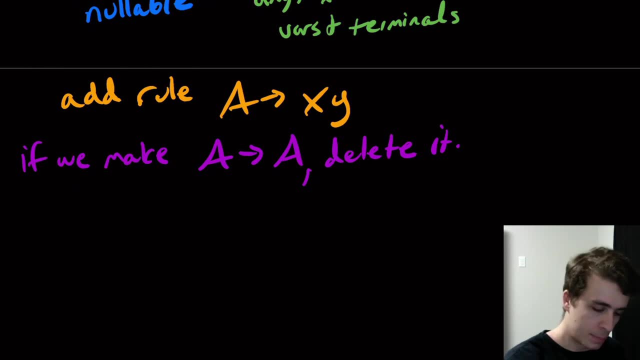 to empty this rule doesn't do anything, so we might as well just delete it. it's not going to actually help us, it's not harmful, it's just that it's not going to help us at all. okay then, and then in the case that the start variable is nullable: 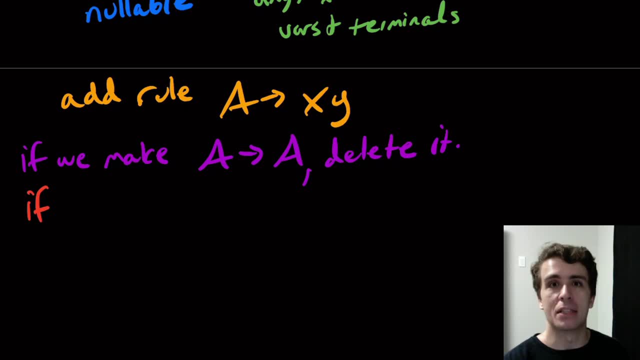 we got to add that rule to allow it to make this the empty string. so if the start variable is nullable, then we add the rule as zero goes to empty, because if it's nullable it can make the empty string. so we gotta not change the language. so we better add that rule at the beginning. so that's just a side case. 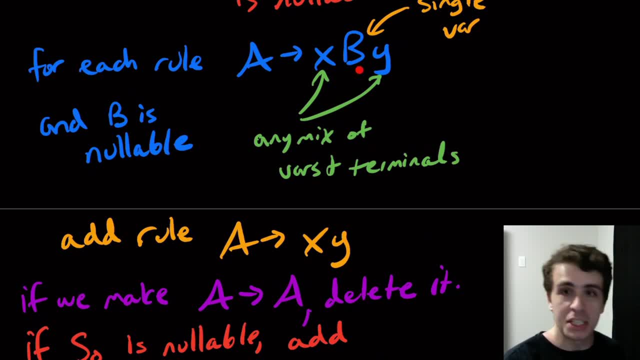 but the main takeaway here is that we're simulating a nullable variable with another rule. we're adding a rule, so why does this rule give us this nullable rule? does this not change the language of the grammar? If we can make the empty string clearly, this is: 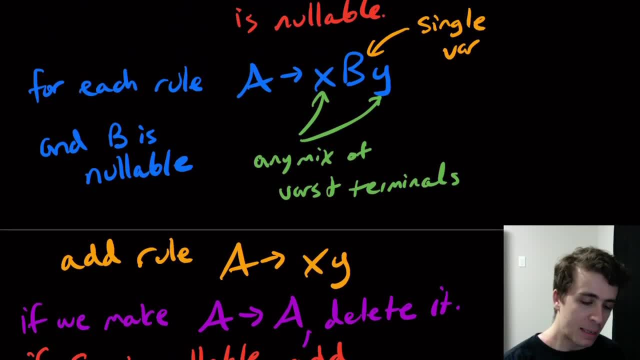 going to still make the empty string, so that doesn't change. But in the case that we don't suppose that we applied this rule and b went to empty, then we can go through this rule instead in the new grammar, going to it directly, And then if we had this rule, then we can reconstruct. 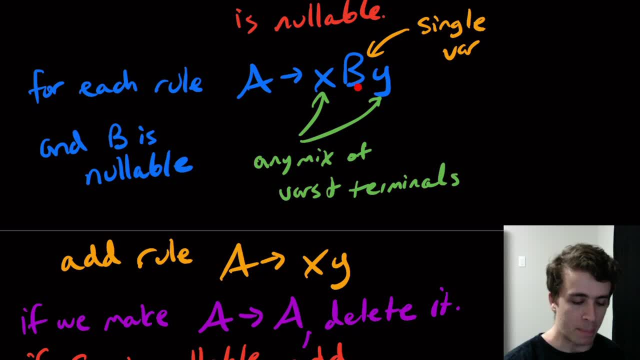 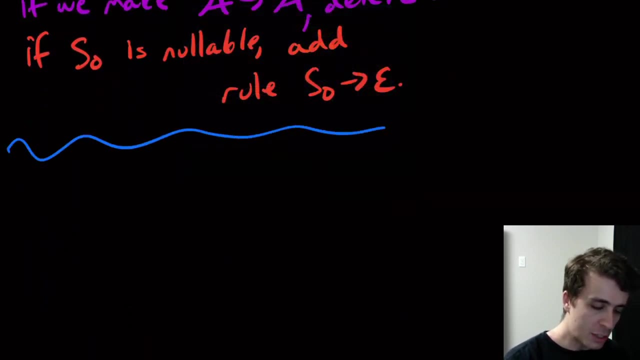 the derivation in the original one by choosing this rule instead and having b go to empty instead. So that actually proves that this doesn't change the language of the grammar either. Okay, cool. So and one thing to note here is that the order of these rules, these steps, that we're 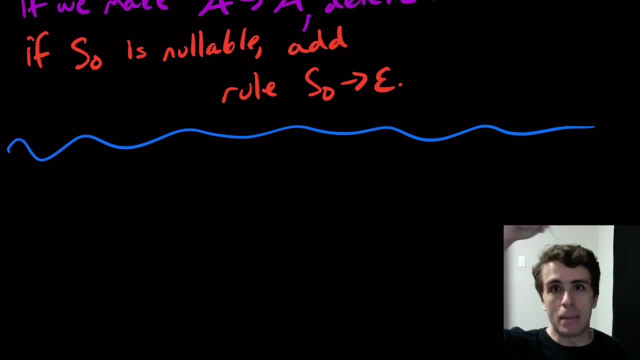 doing are actually important. What I actually recommend you trying to do in the comments is: do the rules in some other order, The steps that we do in a different order. Does it always work? And it turns out that it doesn't. but I want you to find a counterexample to show that changing the order of the steps actually 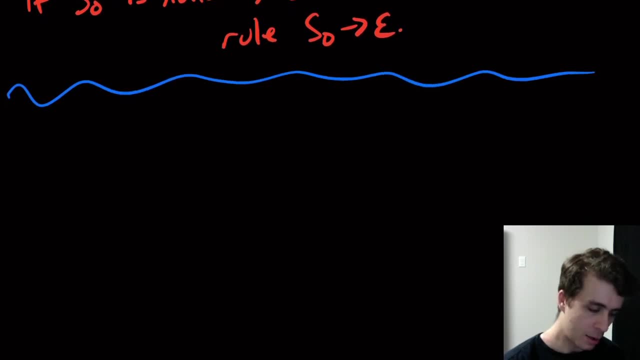 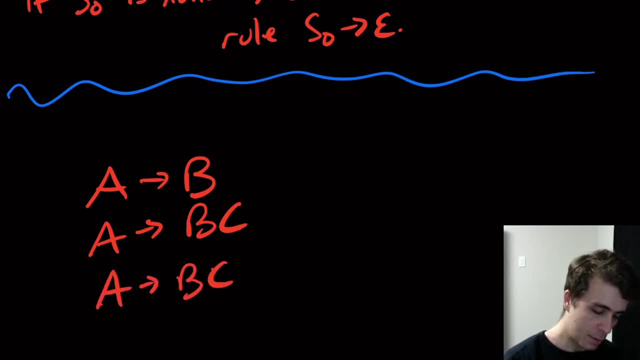 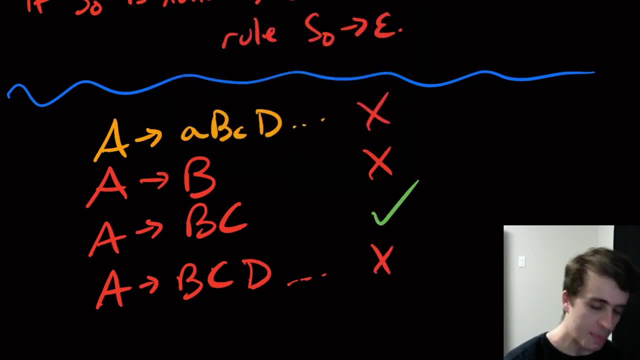 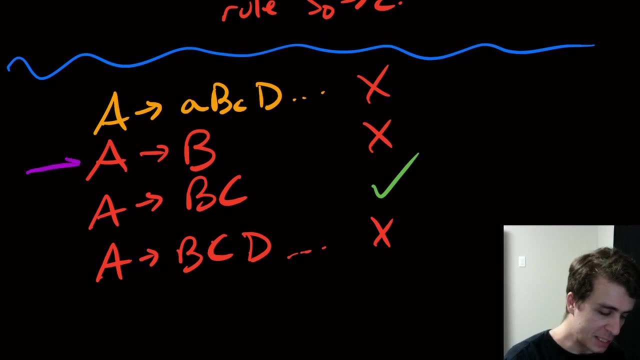 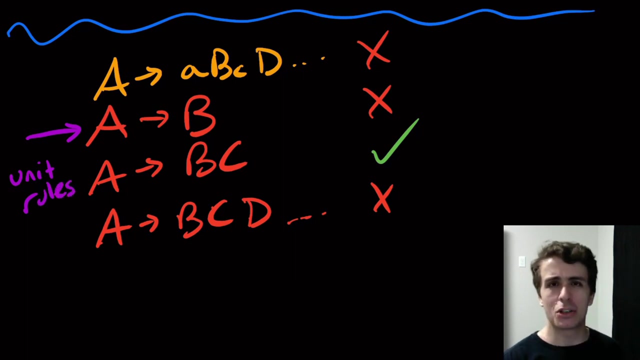 this: get rid of the fourth one and keep the third one, because it's okay with Chomsky, normal form. So the one that we're going to deal with next is this, This one. So these are what are called unit rules, And in some sense they're kind of useless. 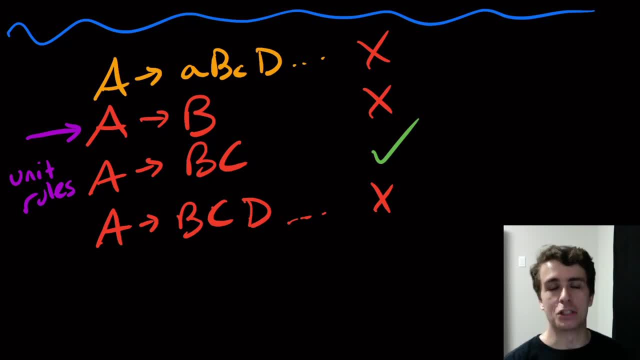 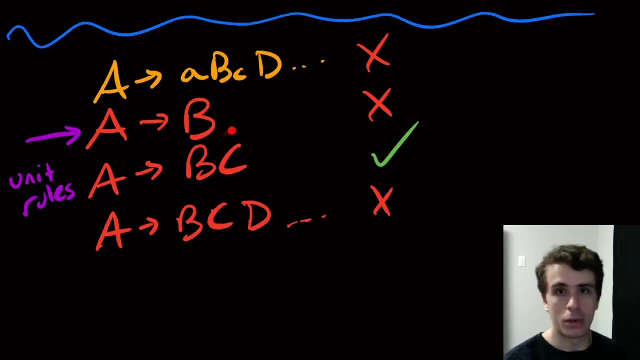 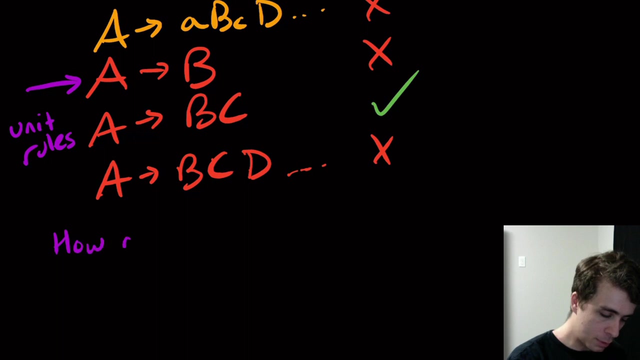 because they don't actually make anything of the string. They're just changing one variable to another one, right? They're not producing any terminals, They're not doing anything else other than going to another variable. So the question is: how do so? this is the third step. how do we? 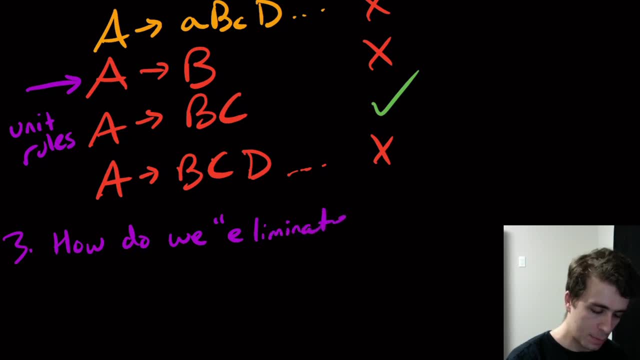 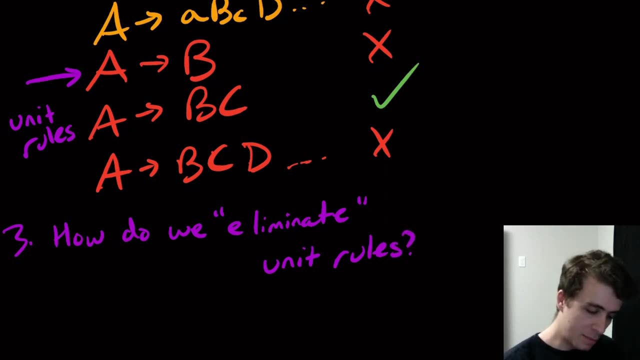 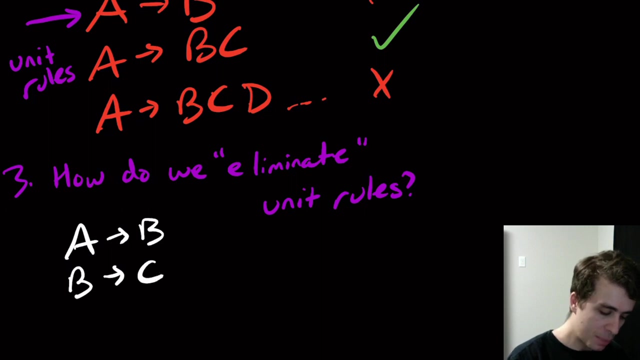 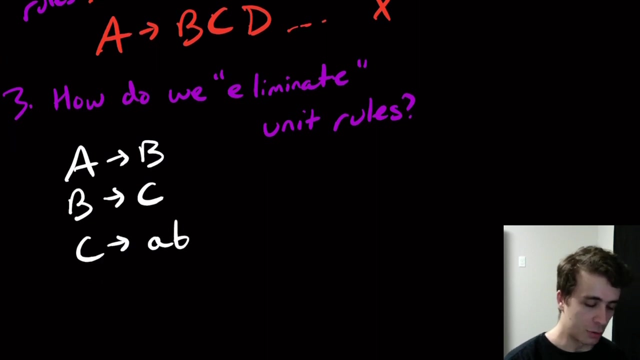 quote unquote. eliminate unit rules. So let's actually motivate this with a small example. Suppose that we had like: A goes to B, B goes to C, C goes to, let's say, little a, and that's it, or AB or something, So some string of terminals down here. Well, what we notice is that A can. 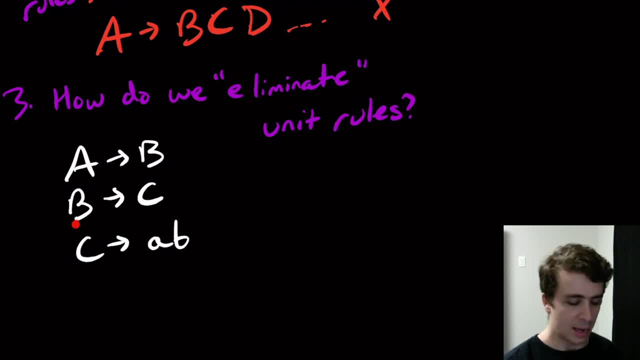 also make this string of terminals AB, and also this variable B can make it too. So the way to fix this, or one way to fix it at least, is to have A make AB, the variable B also make it and C also. 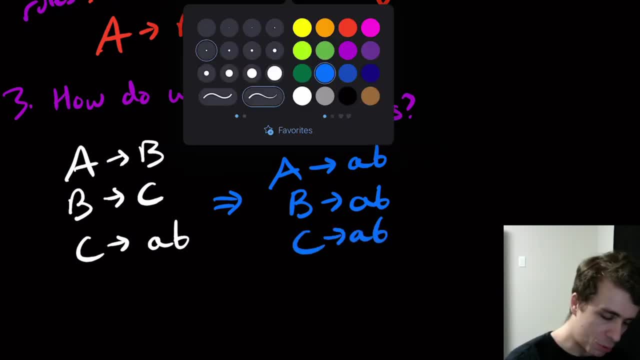 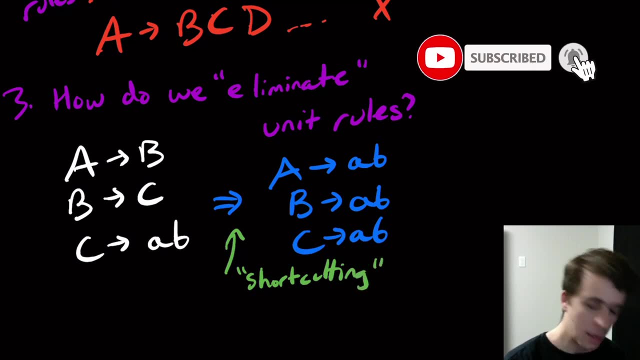 make it So in some sense, what this process is doing right here is we're shortcutting right. So if you think about a chain of unit rules, we're basically just shortcutting our way down to, eventually, where we get something that isn't a unit rule. Keep in mind that these variables, like 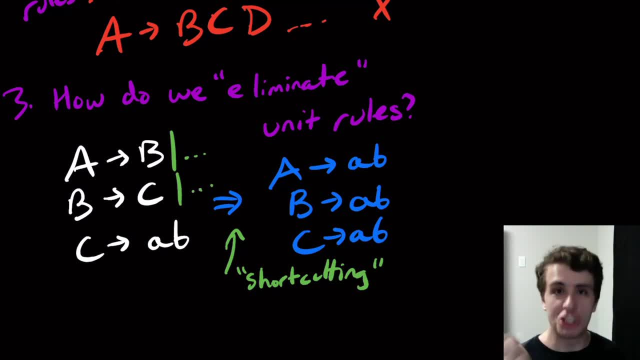 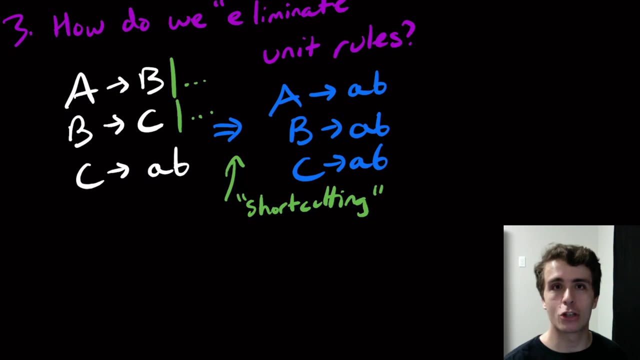 a and b could have other stuff too. So it's not that it's just a unit rule. it's just that there is a unit rule And we want to obviously eliminate them. So here's how you actually do this, And this is not actually taught correctly, So I want to actually correct the record on this. So what? 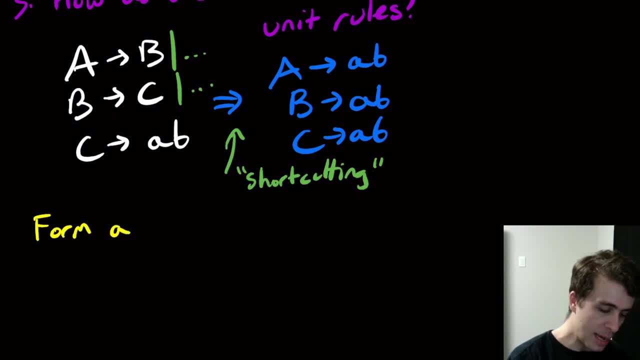 we're going to do is we're going to form a directed graph And if you happen to not know what that is, it's basically just a bunch of nodes right here and some edges with an arrow, And so it's kind of like transitions in a DFA or something. 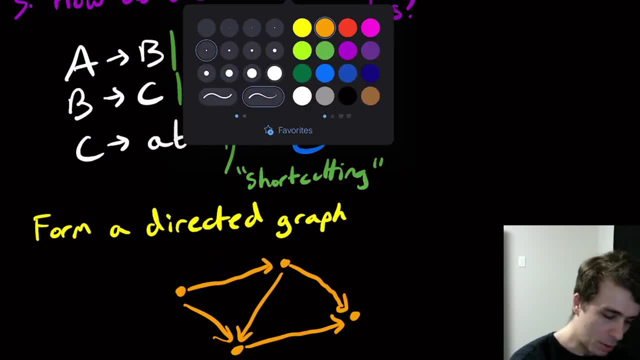 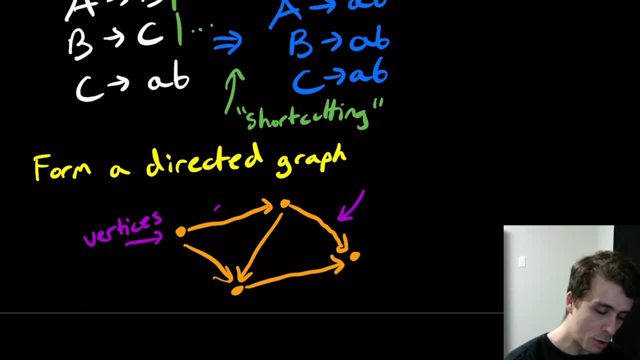 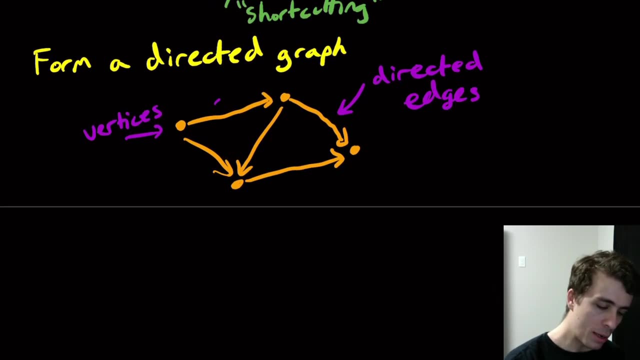 And these are: oh, I shouldn't, I'll mark it. So these here are the vertices, And the arrows are what are called directed edges. So how are we going to form this directed graph where the vertices? let's just do it this way. 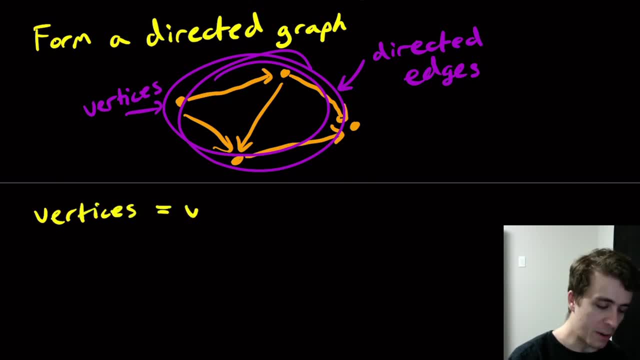 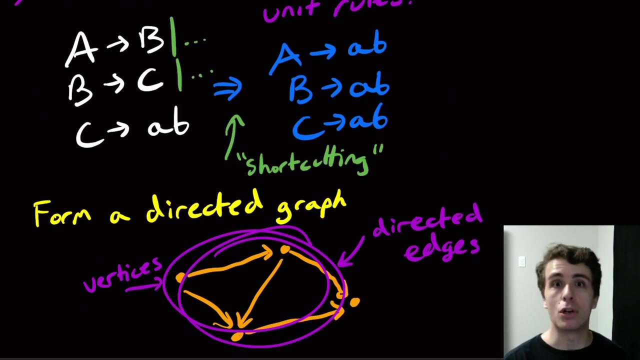 So the vertices are going to be the variables And we're going to form the edge a to b- if a to b is a unit rule. So in the case above we will have three vertices- a, b and c- and then directed edges from a to b. 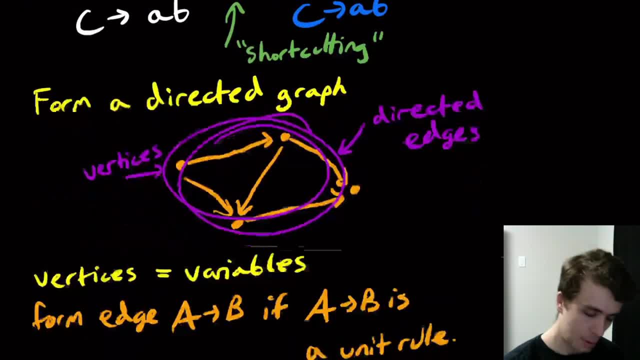 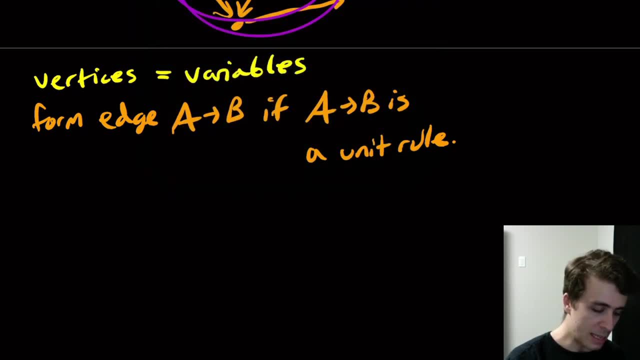 and then from b to c. Okay, So what are we going to do? We're going to form a directed graph. So what are we going to do with this graph? So then, what we're going to look at is look at any pair of vertices- a and b- in the graph. 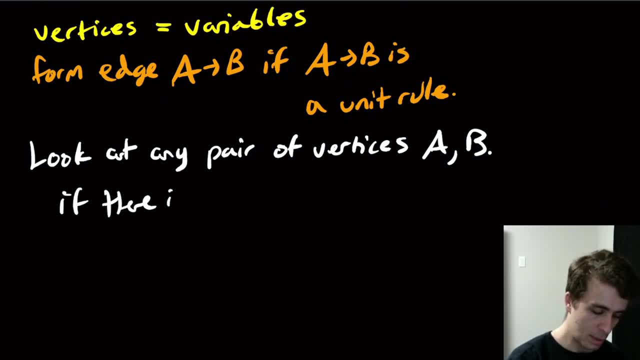 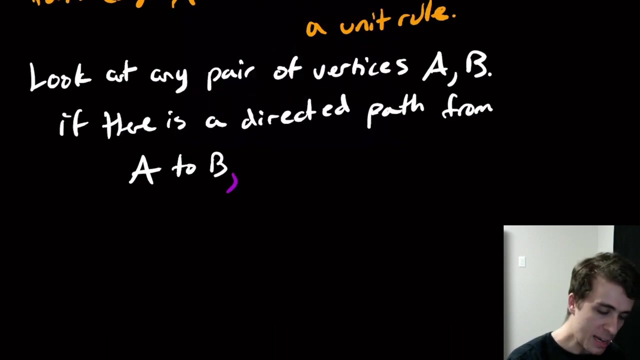 If there is a directed path, so if there is some way from a to b, Okay, So that means that there's a chain of unit rules to eventually get there. So then what we're going to do if that's the case, look at all rules of the form a goes to: 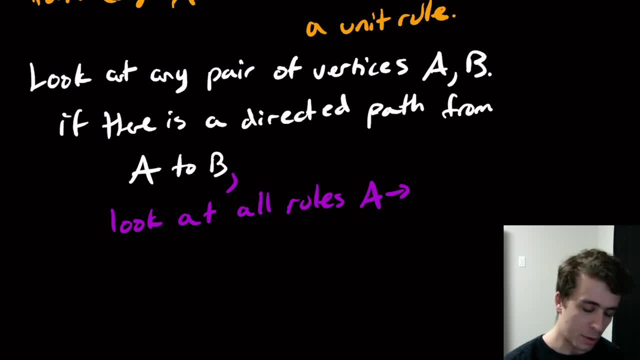 okay, yeah. So if that's the case, we're going to look at all rules that happen to have okay, yeah. So if that's the case, we're going to look at all rules that happen to have Okay. So we're going to look at all rules that happen to have an a inside them. 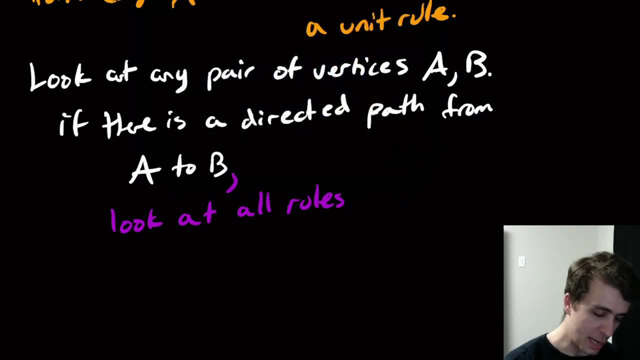 So let's just say that that is something that looks like x is a variable which goes to something. let's give it a name. so let's call it alpha capital, a little beta. So this is okay. yeah, So if that's the case, we're going to look at all rules that happen to have an a inside them. 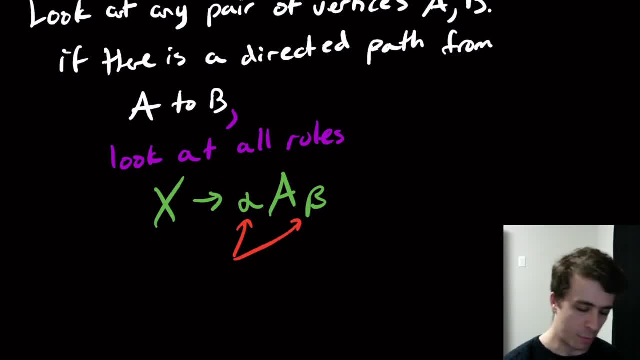 Okay, So we're going to look at all rules that happen to happen to have an a inside them. alpha and beta, just like x and y were before, are a mix of variables and terminals. so look at all rules of this and then what we're going to do is we're. 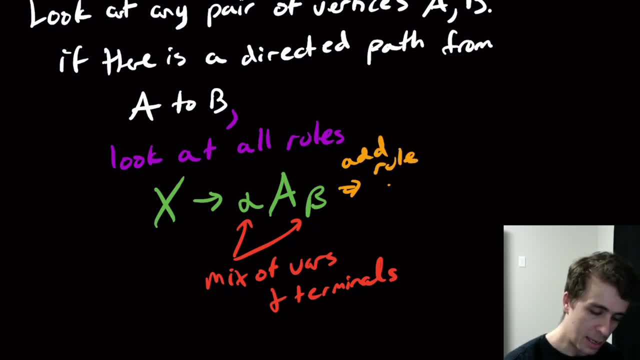 going to add. the rule x goes to alpha, B, beta. okay, so in some sense we're adding this rule right here to shortcut the way from A to B, because there's a chain of unit rules that takes us from one to the other. whoo, so why does this actually not? 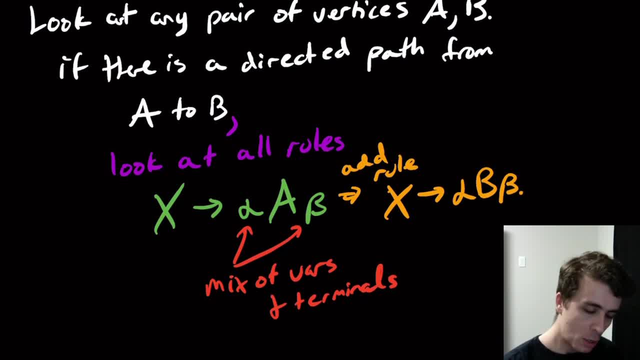 change the language of the grammar, because we'll think about this. if I apply a sequence of unit rules from A to B, then I could have just applied this rule right here, okay, so then what about the other way? so let's just say that, um, um, I applied this rule right here. what you can do again is reconstruct the. 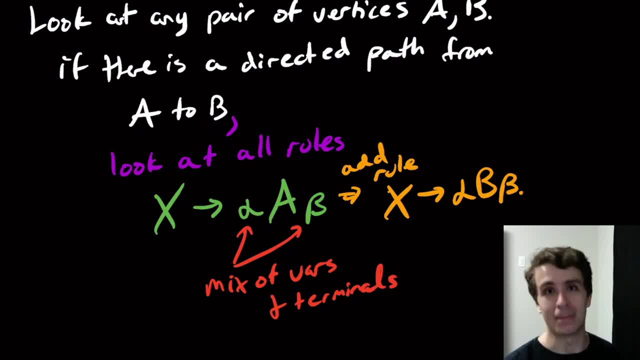 sequence of unit rules that it took to get from A to B. okay, so that actually shows us that, that it actually works. if this is a rule that was created and it was used, that means that there's a sequence of unit rule applications that got us to this, because this is the rule we added. so then look at the one of the. 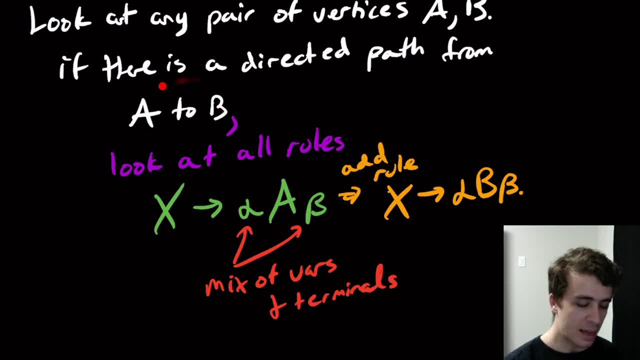 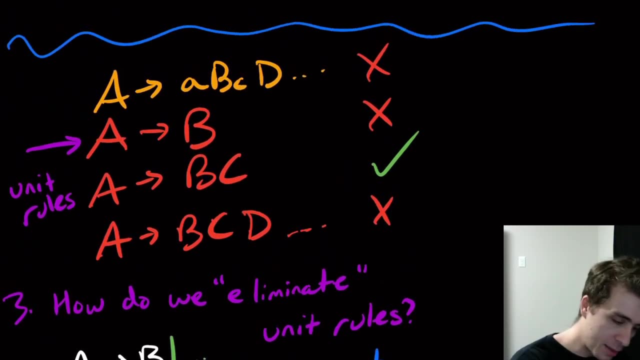 ones that was created before then. if, then, that must correspond to a path in the original graph, and then correctness follows from that. okay, cool, so that means that from here we have finally fixed this rule type right here. I'm gonna leave an X here to indicate that that was a problem before, but the purple check mark means that we actually 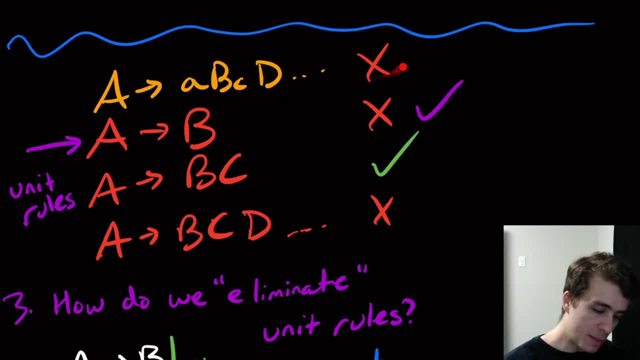 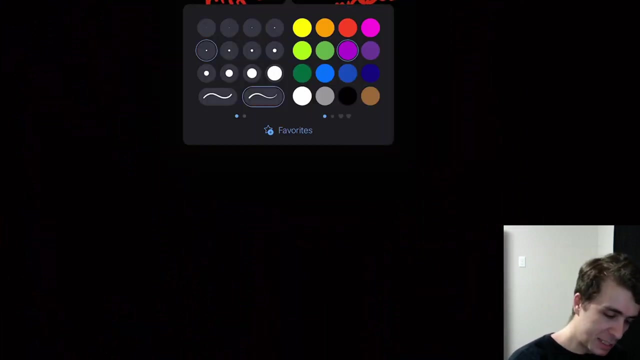 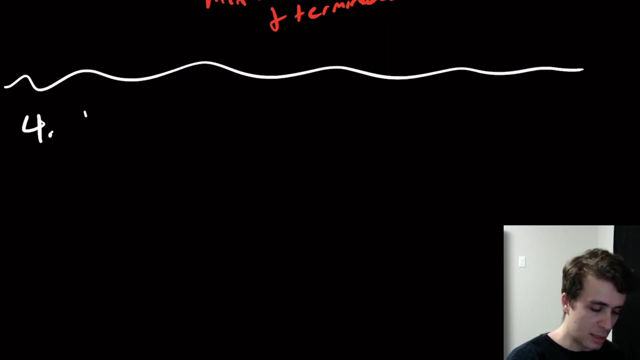 fixed it, okay. so then what about these two right here? so what we're gonna do is the, the last little bit. they're all. there's only a little bit more in stages, in two stages. so let's handle the one where we have a mix. so let's say: let's, let's break up the mixes, the mix of variables. 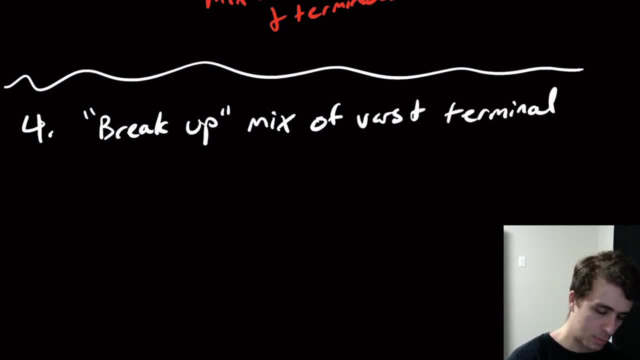 and terminals. so what we want to have here at the end is to have a variable that makes a single terminal, or a variable makes a bunch of variables. so all of these right here are variables. that's not in Chomsky normal form yet, but it's really. 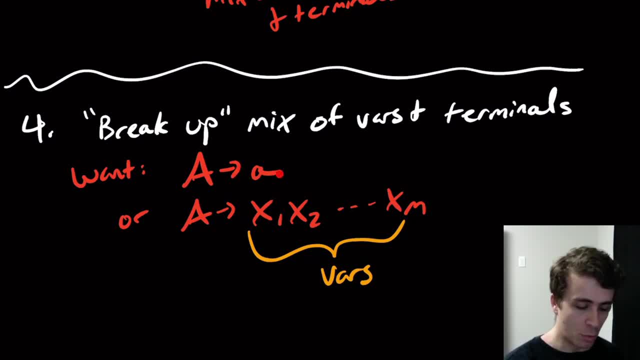 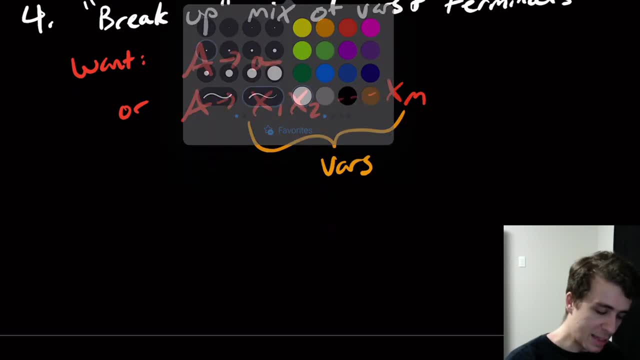 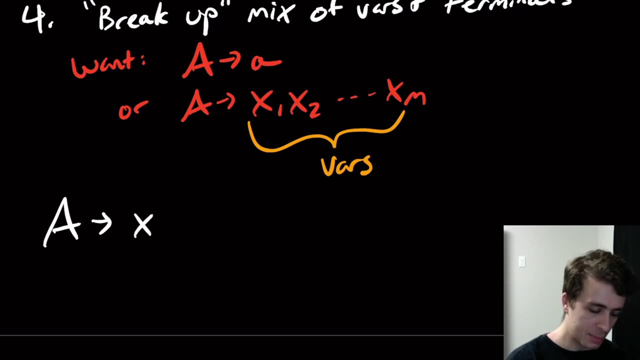 really close here, so it's the one. one terminal is good. it's just that there may be a lot of variables. so let's just look at the case of where we have a variable. a is going to make X, a little a Y, so here I'll do it in green. so X and Y, just like before, are a mix of. 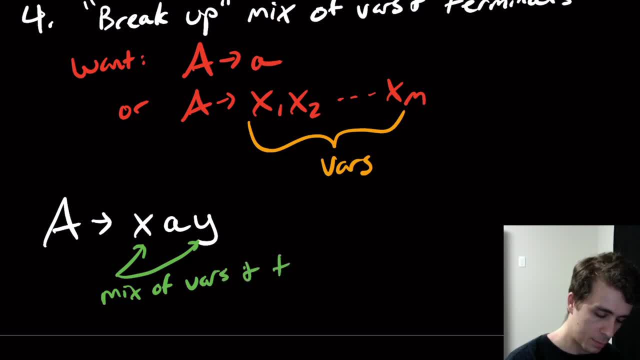 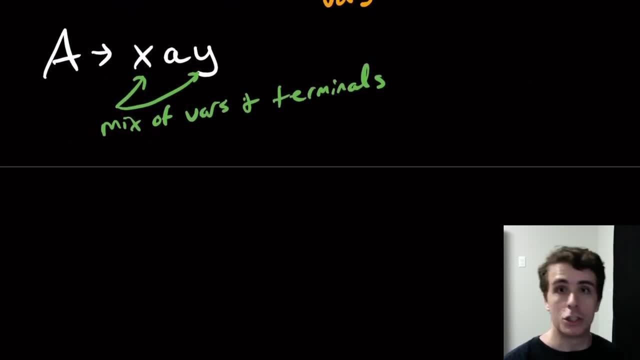 variables and terminals. so what do we actually want to do here? well, what we want to do is to replace this terminal with a variable, and normally you can't do that. but here's the trick. what we're going to do is to add a new variable. I'm going to call it u sub a, and it's only rule for it is to 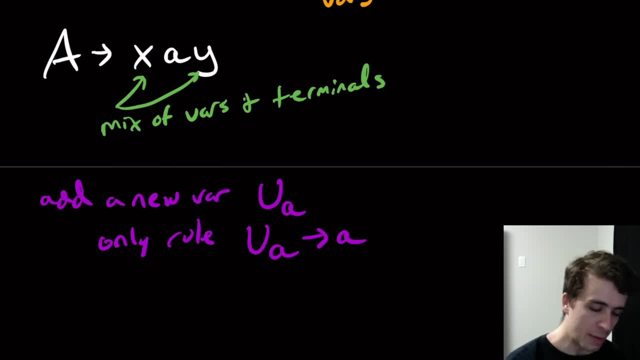 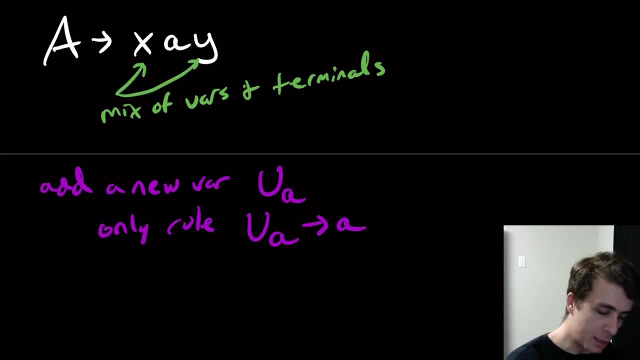 make the corresponding terminal. so whatever is in the subscript, that schongefゲ ok. so then what we're going to do here is to replace. we're going to replace that rule x sei, not just add the rule. we're going to outright replace it with a: goes two x u. 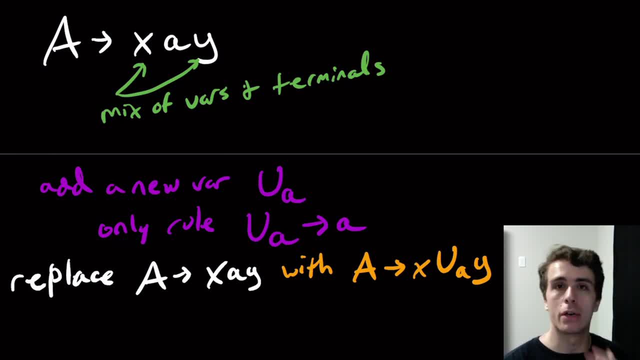 sub a y. so in some sense we're going to convert all the, the terminals, into variables. The only thing that we want to require here- and there's a very good reason for this- is that the length of x and y together is at least one. 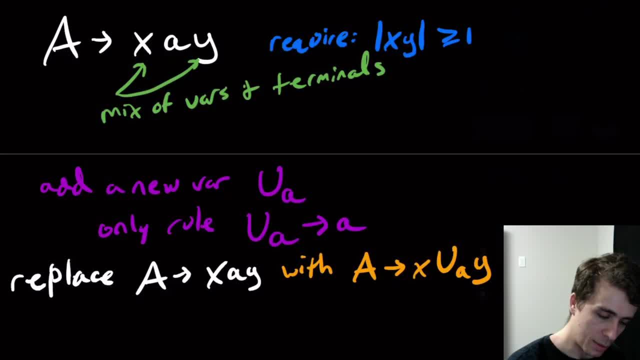 So let me turn off, okay. So that means that x is not equal to empty string or y is not equal to the empty string. Why is that the case? Because if they were both the empty string, that means that this variable a only made a single terminal, and if we replaced it with a variable, 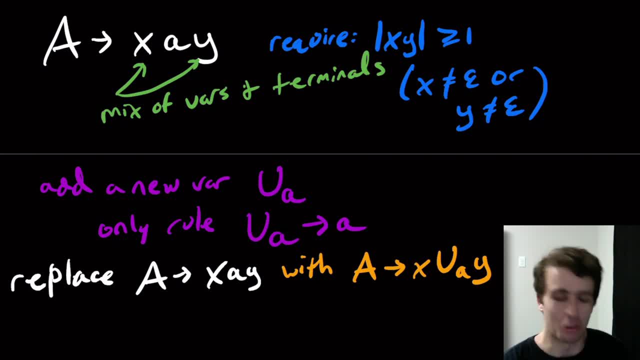 then we just made a unit rule and we just got rid of unit rules And and so the if it was just a single terminal over here, that's not gonna. that's correct for Chomsky Normal Form, so we don't need to do anything about it. So if one of the two have something, then we think. 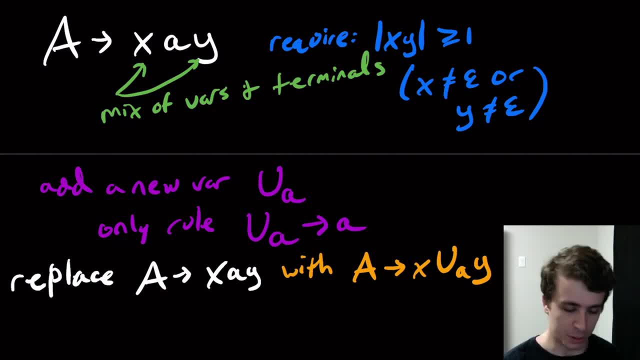 we're going to be able to do something about it. So if one of the two have something, then we think do want to convert it into variables, So we do want to do this procedure. But yeah, so we're all we're doing is we're converting a terminal in a longer right-hand side into a variable. 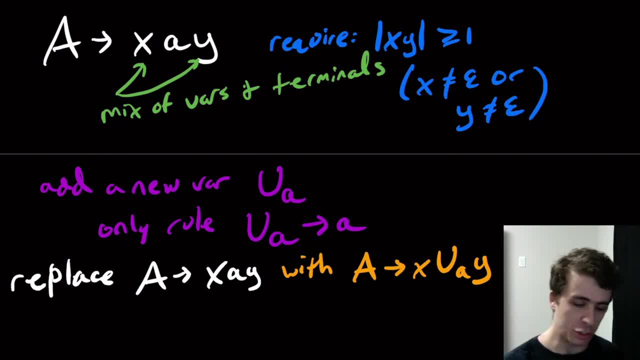 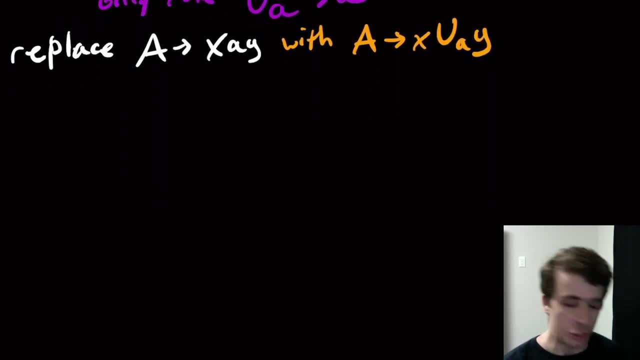 So at the end, we have either a single terminal, which is enforced by this up here, or we have a bunch of variables. So then now the only thing we need to do is to break up those so-called right-hand sides that are long. So the fifth step is to 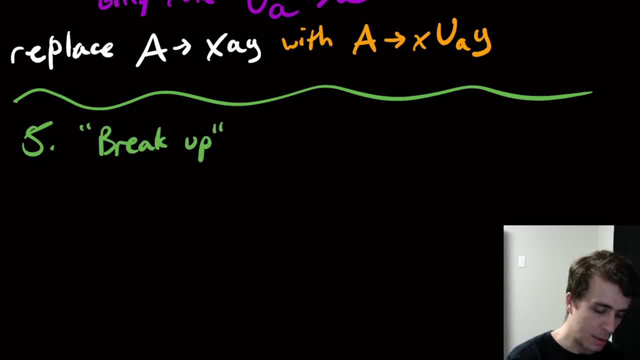 break up. what are what I call long right-hand sides? And what does long mean in this case? It means the length is at least three, So why not one? Well, if it's one, then it's a single terminal and we can't break it up. If it's two, and we don't have unit rules, so we don't have. 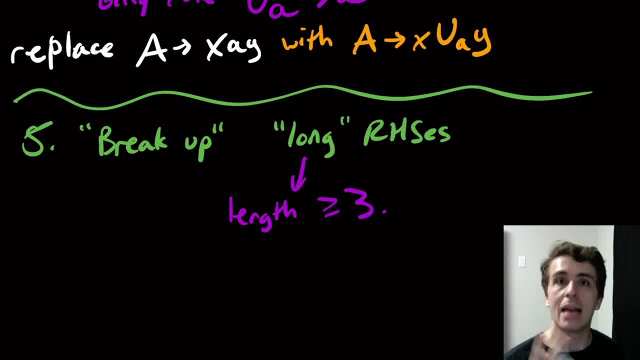 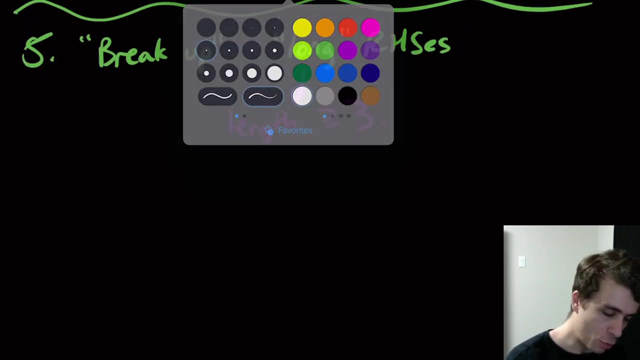 to worry about that. If it's two things, it can't be two terminals, because we just figured that we could fix them. Otherwise it's two variables and that's okay for Chomsky normal form, So it's of length at least three that we need, Okay. so let's say that we have a really long right-hand. 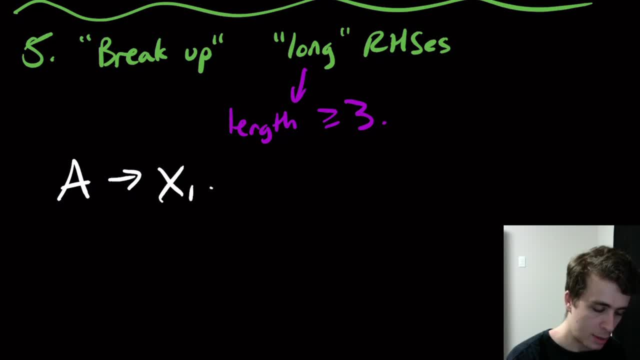 side here. A goes to x1, xm, and we have to. we should remind ourselves that all of these are variables And, of course, for this to actually make sense, m has to be at least three, which is a number of variables over there. So what can we actually do here? This is actually a pretty cool. 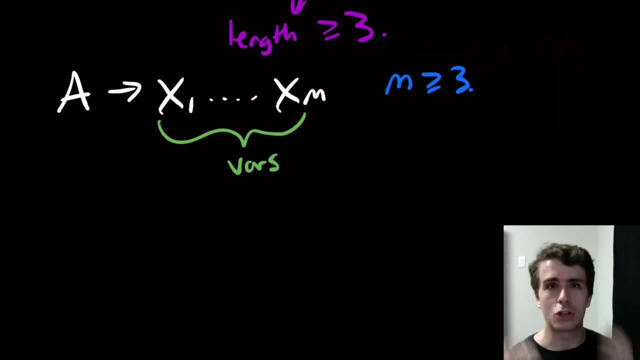 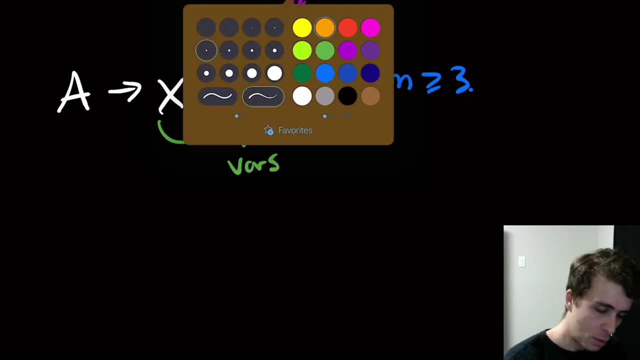 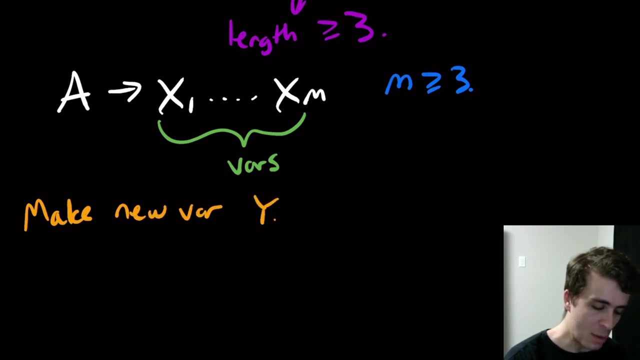 trick, and it's actually kind of hard to see if you try to get an intuition for, but it actually makes total sense once you see it. So here's the idea. What we're going to do is to make a new variable- I'm going to call it y1, and what we're going to do is these two rules. 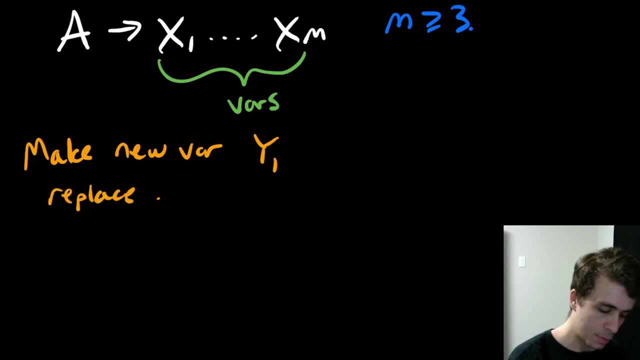 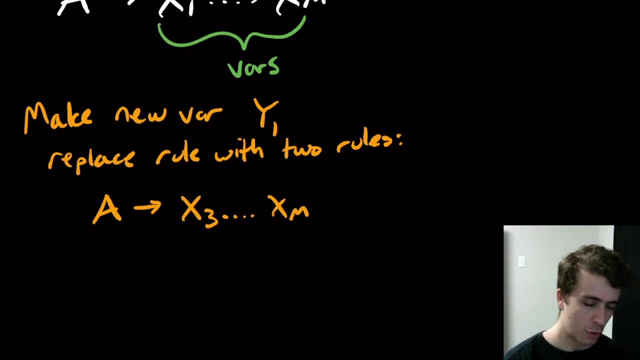 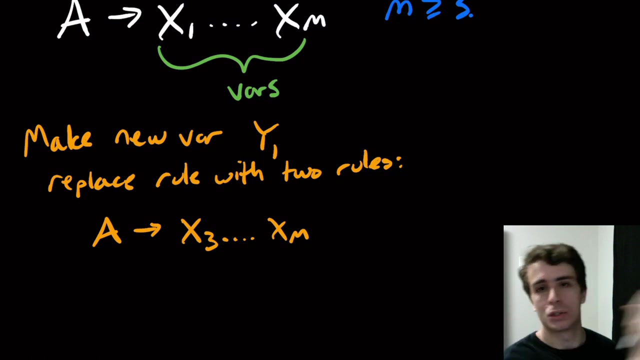 So we're going to replace that rule with two rules. And what are those two rules? It's going to be a goes to x3, up to xm. There are actually multiple ways you can do this, but this is just one way. a goes through x3, that's why we said there is at least three variables: up to m And. 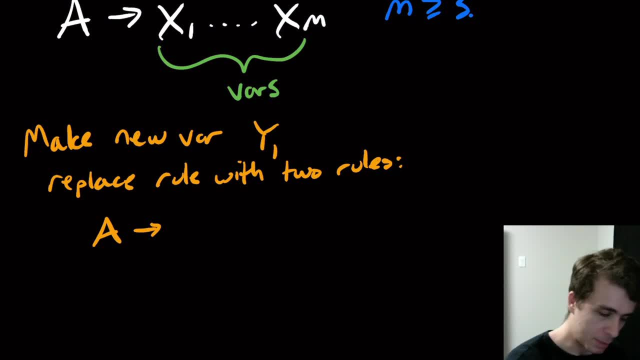 actually no. no, sorry, That was my mistake. It should be y1, x3 up to xm And y. maybe I'll do this in a different color. So y1 is going to make the first two variables. Okay, so in some sense we're taking off the first two variables, sticking them with this. 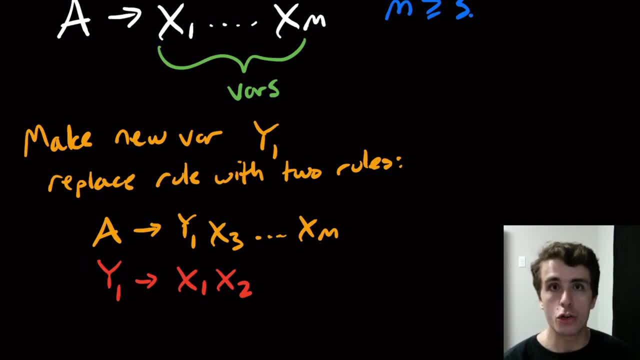 brand new variable. So it has to be a brand new variable every single time and I'll explain why in a sec. So brand new variable makes the first two and I'm sticking that variable where those two variables would have been x1 and x2.. They would have been here, but I'm essentially just 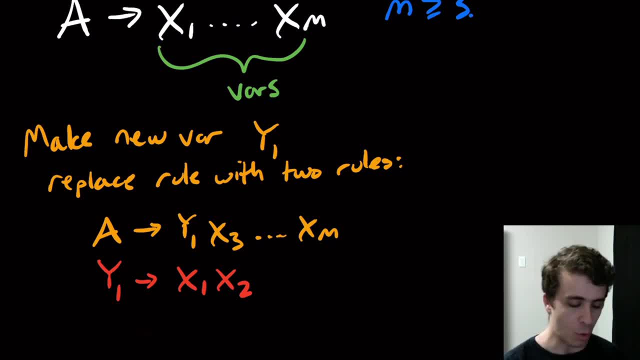 replacing this with y1.. And what we can notice is that right here we have m minus one variables, So it's a smaller problem than we had before. We had m before. now we have m minus one And this, this rule down here, is okay because we have two variables, which is okay for Chomsky Normal Form. 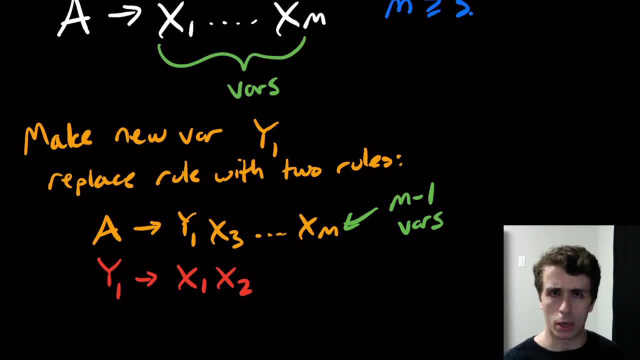 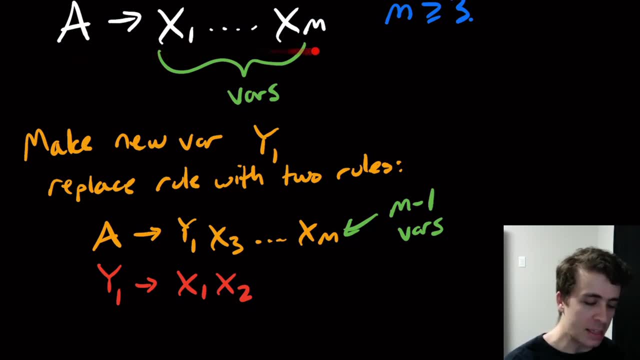 Okay, so correctness. Why does this work? Well, intuitively, once you see this, it works. But let's actually think about this: If we applied this rule in the original grammar, then in this grammar we have to go through y1, and because y1 is brand new, this is the only rule. it. 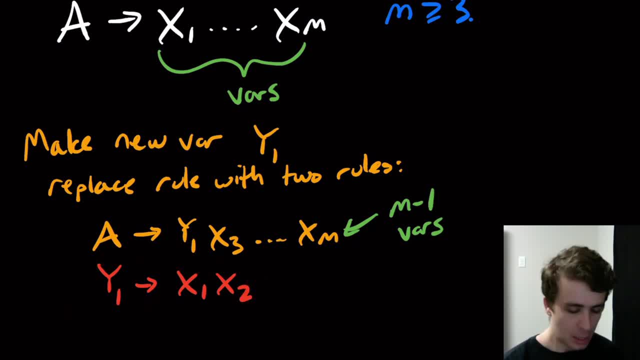 corresponds to, It doesn't have any other rules. So it must do x1 and x2, and those will be replaced right here, because I have to replace y1 with something and it has to be replaced with x1 and x2.. So again, it simulates the same rule that we had before. So what about in this grammar? 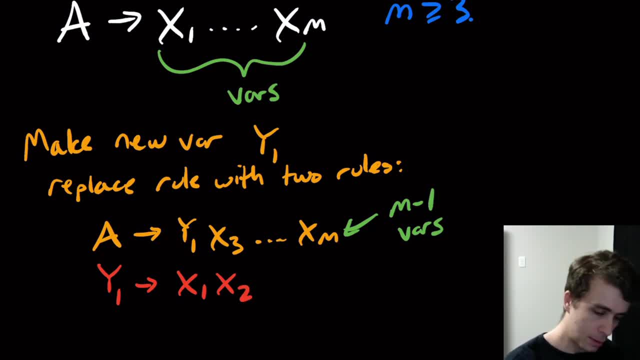 Um, oops. So if I apply this rule- sorry, if I apply this rule- then do I get the same original rule in the original grammar? And the answer is yes, because I have to apply this y1, and it's replaced with x1 and x2, because that's the only rule it corresponds to. So, in fact, 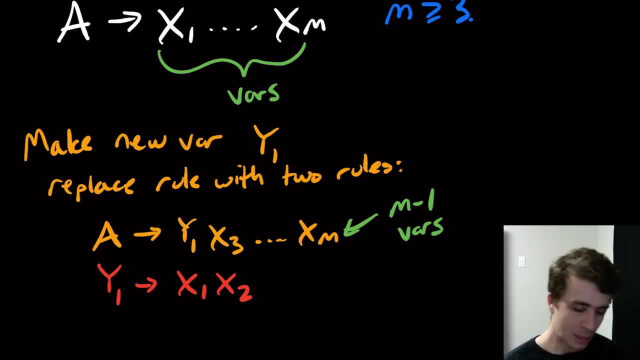 this gets exactly the same language yet again. So the cautionary tale is that this y1, must be brand new. It can never be used for any other rule. It could in practice, but for correctness to work for every grammar this, you have to be able to show that it can. 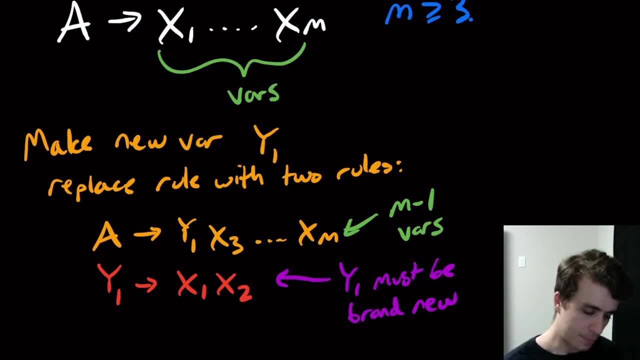 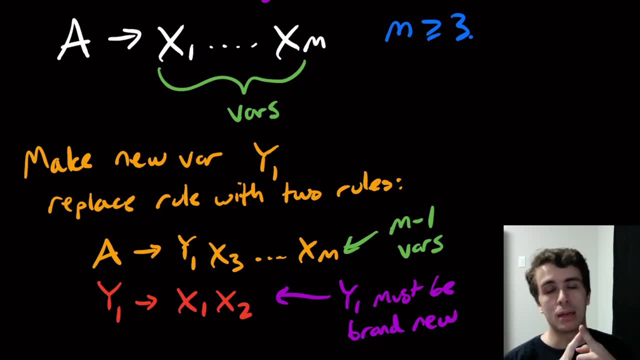 never be used for any other rule. Okay, so do we have something in Chomsky normal form? Well, the start variable is the only variable that can make the empty string. because we've enforced that There's no unit rules. We got rid of them, And this step along with all the others. 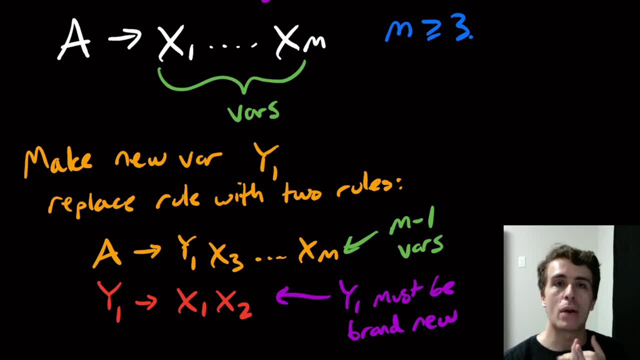 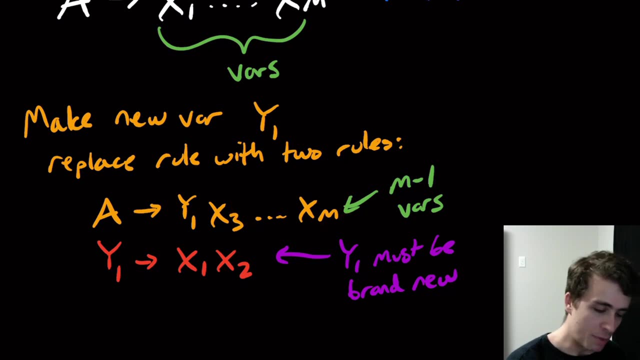 doesn't introduce unit rules. We don't have a right-hand side that's mixed of variables and terminals, because we got rid of that in step four. We don't have a long right-hand side because this step actually breaks it up. Now you notice that this has m minus one variables. 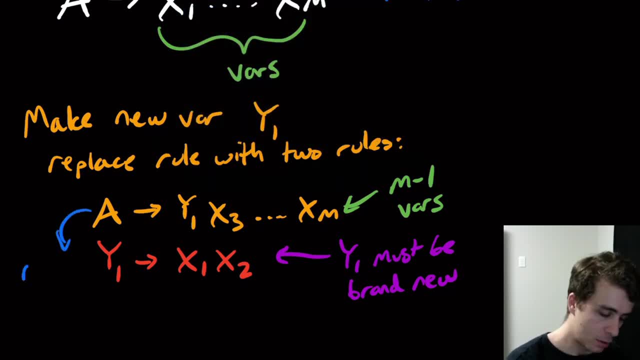 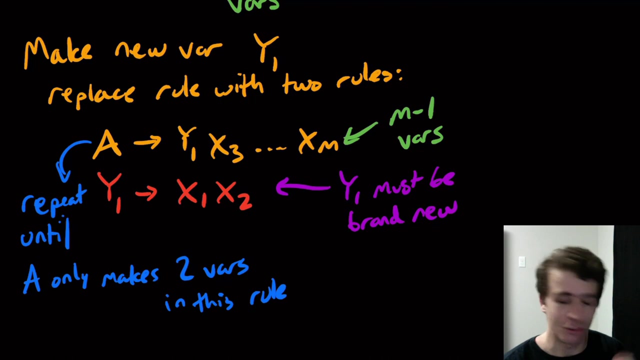 What we have to do is to repeat. So we have to repeat until a only makes two variables in this rule. Okay, so it doesn't make any sense to continue this once it gets below two variables, because you shouldn't get below two, But once it gets down. 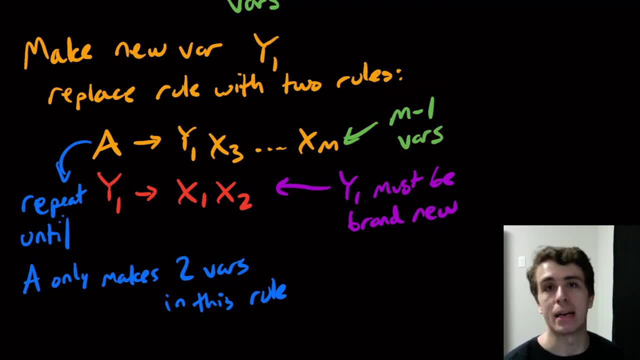 to two, and because we're subtracting by one here, we'll eventually get down to two because m is at least three. So if we actually do this and repeat until we get to two variables, that actually gets us a grammar in Chomsky Normal Form. 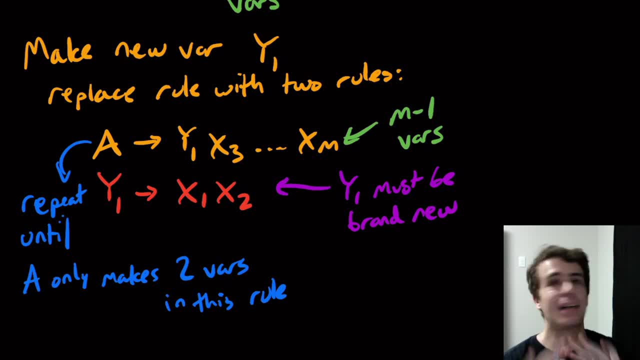 And note: we started with an arbitrary, context-free grammar. I didn't assume anything about the grammar at all. We didn't know anything about its variables, its terminals, its rules or what its start variable is, And so therefore, that proves that every grammar can be converted into Chomsky. 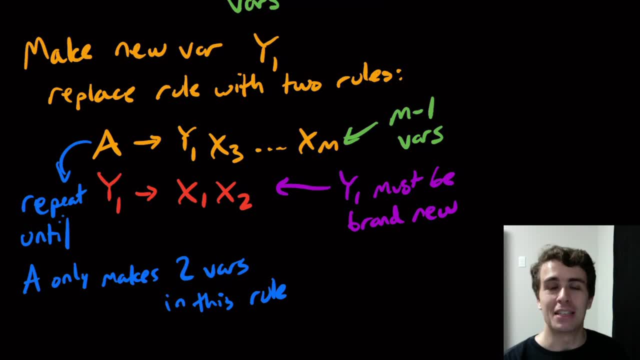 Normal Form Isn't that cool, So hopefully that was interesting. Leave your thoughts about Chomsky Normal Form into the comments. We'll do an example at some point. There are many other links in the video description if you want to support the channel, such as liking.